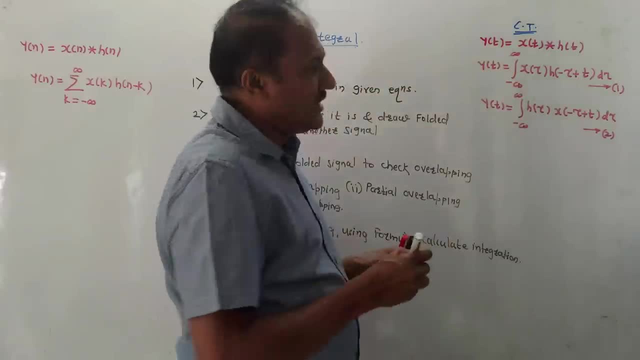 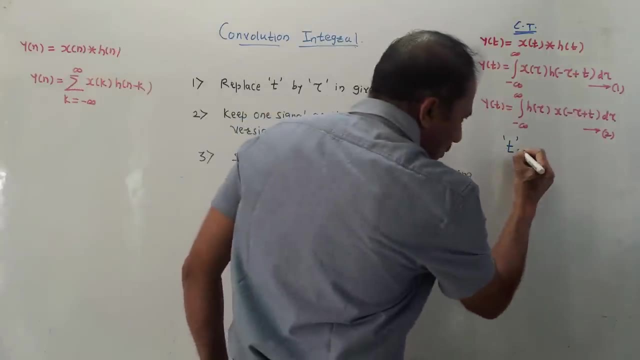 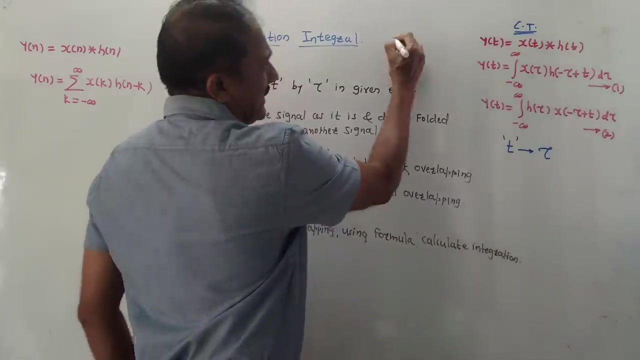 integration: a minus infinity to plus infinity. And one important thing to remember: normal notation. we use t in continuous signal. t stands for time period. If it is convolution, then you will be using new notation, tau. This is the new notation. Like in discrete case we have n In discrete. 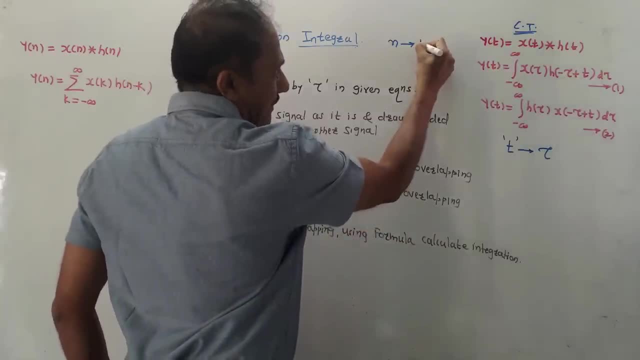 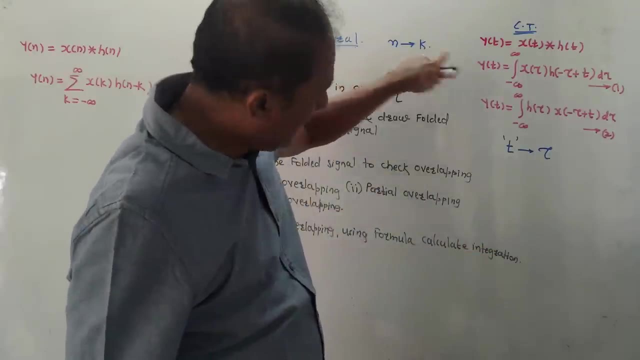 basic notation is n. If it is convolution, then we use k in place of n. If it is monotonous, then we use tau. So whenever you are performing some different operation like convolution or discrete, we have to use k. If it is continuous, we should use tau. 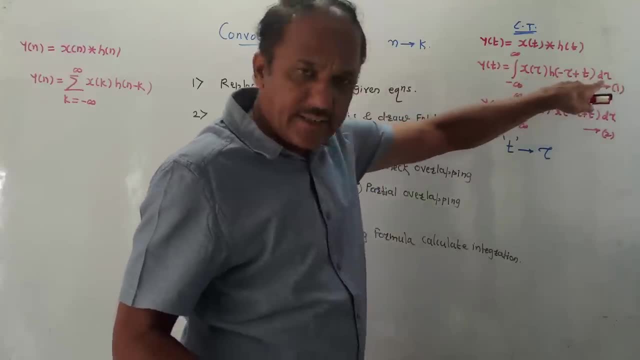 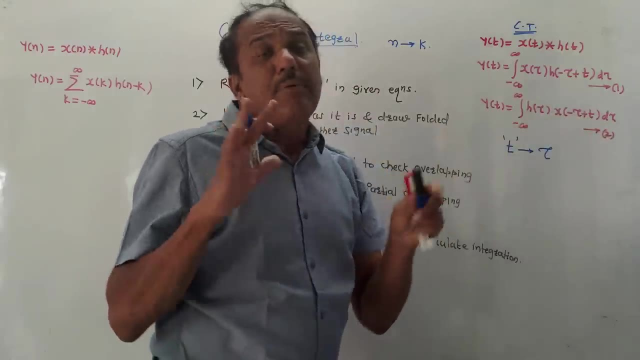 So these are the two formulas: integration minus infinity to plus infinity, x of tau, h of minus tau plus t d tau. These are the integration variables And the next formula h of tau, x of minus tau plus t d tau. that is equation number two. Now the important thing is: 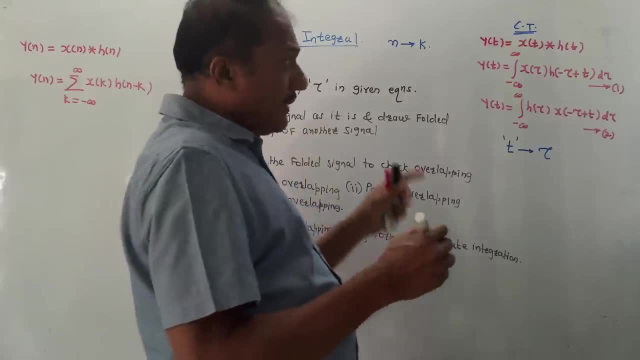 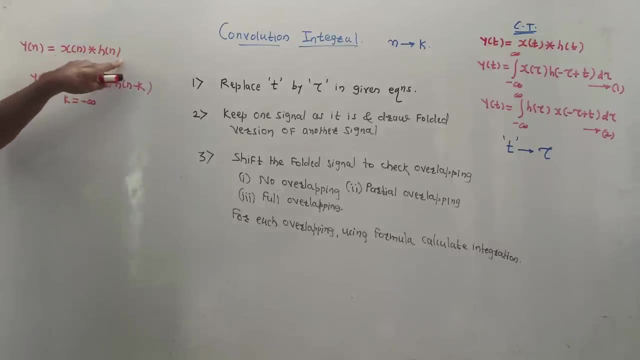 So I will tell you one very important trick to recall the formula of continuous integral. See here: this is the discrete connotation. y of n is x of n, asterisk h of n. This is the formula of discrete convolution. If you think that you don't remember any formula of continuous 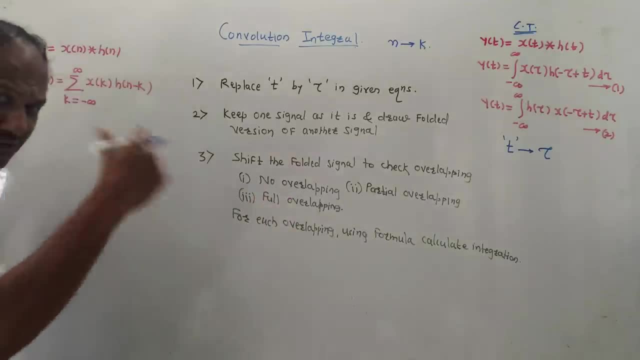 then what will you do? You will use the formula of discrete to prepare the formula of continuous. How will you prepare it? See, in discrete, the notation is n In place of n. we are. this is the notation of discrete. 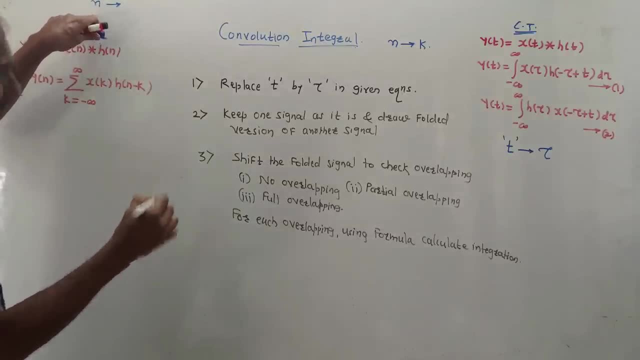 If you think of corresponding notation in continuous, then we use t in place of n. What is the notation in discrete? In discrete convolution, in case of continuous? in continuous convolution, the corresponding notation is tau, Means we have to use tau in place of k. 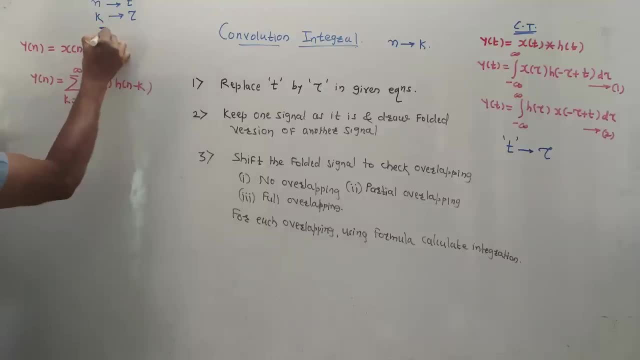 And one very important thing: we always use summation in discrete, We always use integration in continuous. If you remember these three things: in place of n, we have t In place of k, we have tau In place of summation. 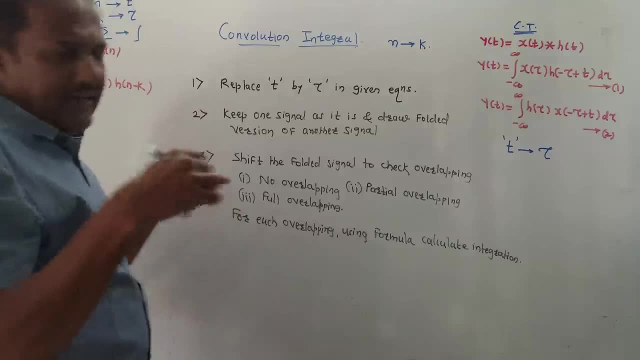 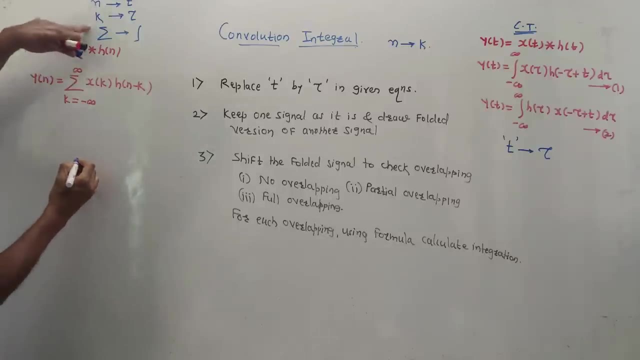 we have integration, You will be in a position to generate any formula of continuous signal Like this is the formula of discrete. I have to prepare the formula of continuous. See here to remember these changes. if y of n is there, then I will be writing y of t. 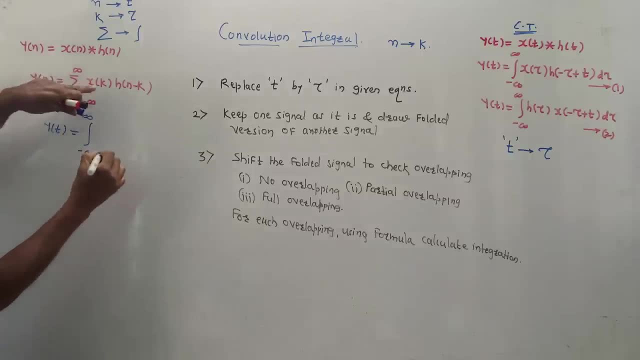 If summation is there, in place of that, integration will come. If x of k is there means tau in place of k, then I will write x of tau. If h of n is minus k, in place of n we have to write t. 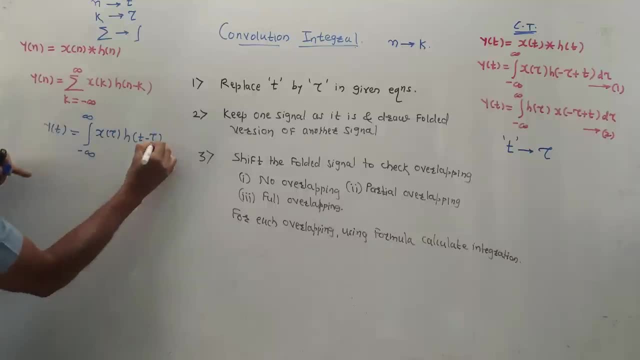 In place of k we have to write tau. If we do integration, we will write t minus tau And for integration we will add the variable t tau, See h of t minus tau is same as h of minus tau plus t. 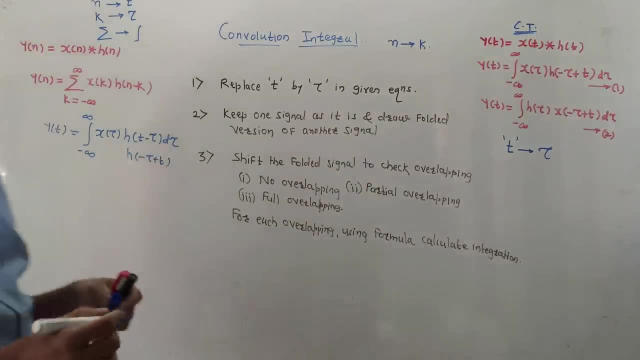 one and the same thing. So with this technique, you can convert any formula of discrete into continuous. Okay, Now what steps do we have to use? In the first step, two sequences are given, Like this: one sequence will be x of t. 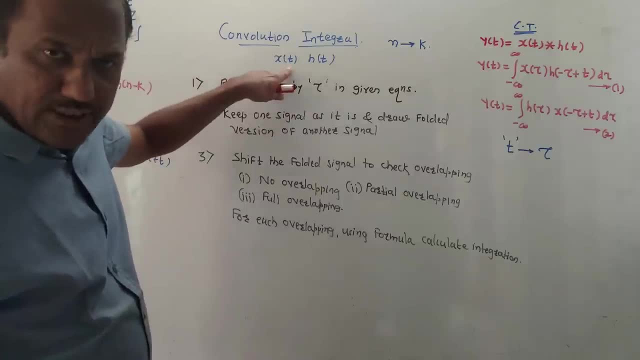 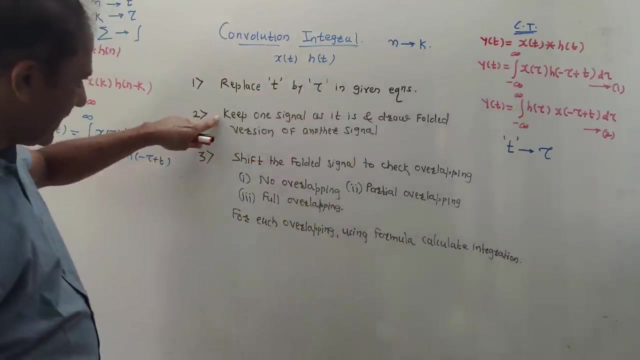 and another will be h of t And it will be asked to calculate convolution integral of these two sequences. uh, first step is replace t by tau in the given equation. second step: keep one signal as it is, for example, like softy as it is right, and draw folded version of another signal. 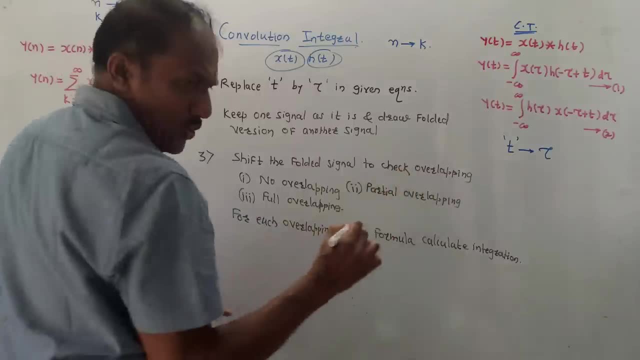 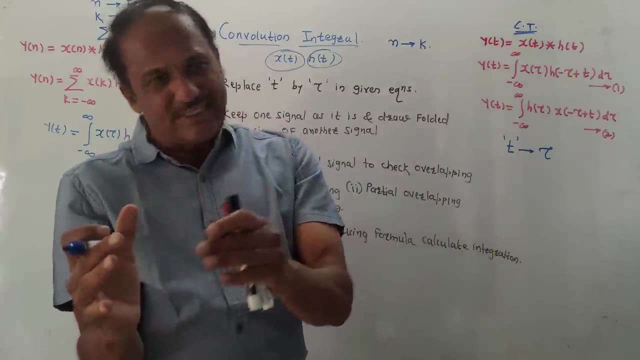 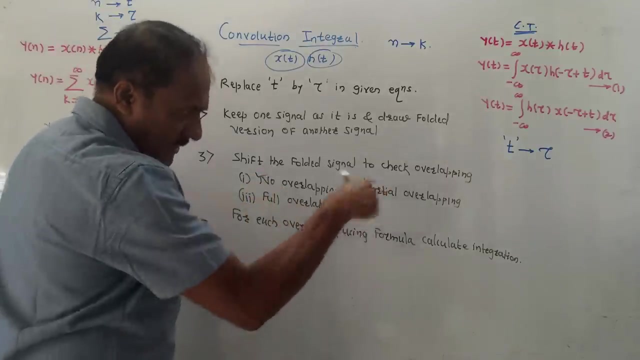 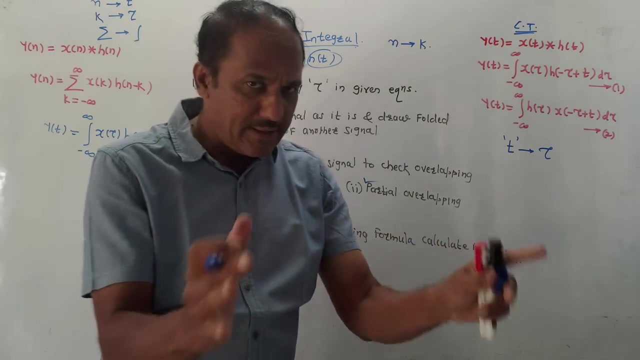 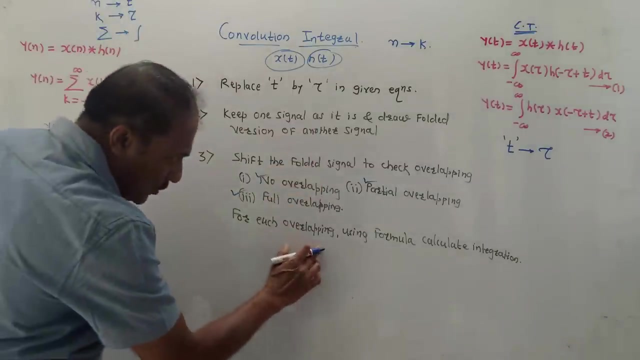 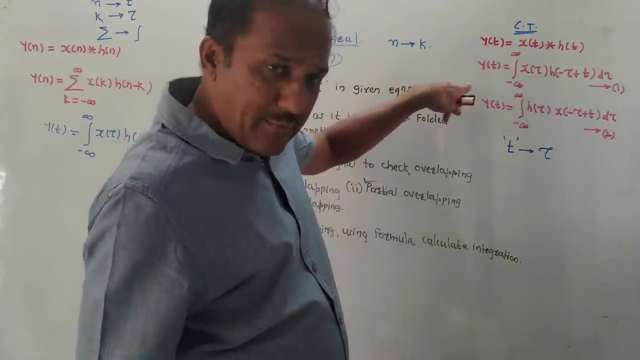 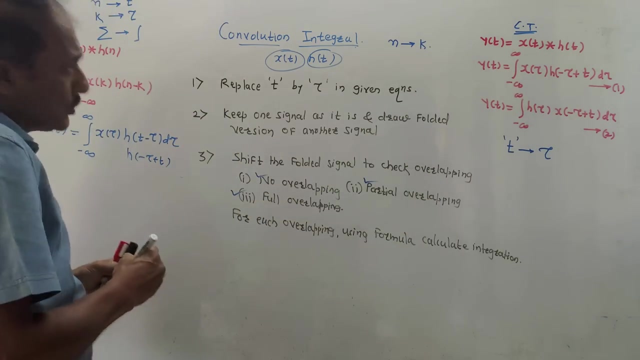 third step: shift the folded signal to check the overlapping shifting. there should not be any overlapping. there should be. second condition, there should be partial overlapping and third condition, there should be full overlapping and for each overlapping using the formula same. there are no rules as such, so, without wasting the time, let us start. 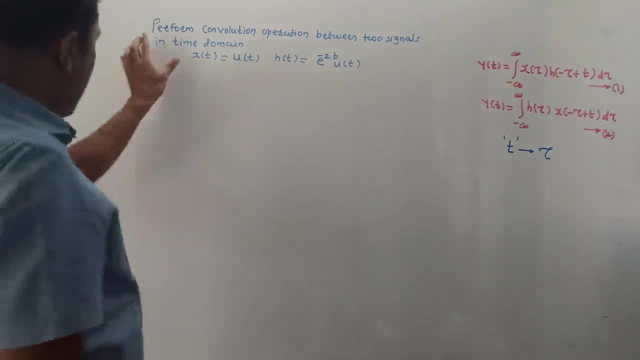 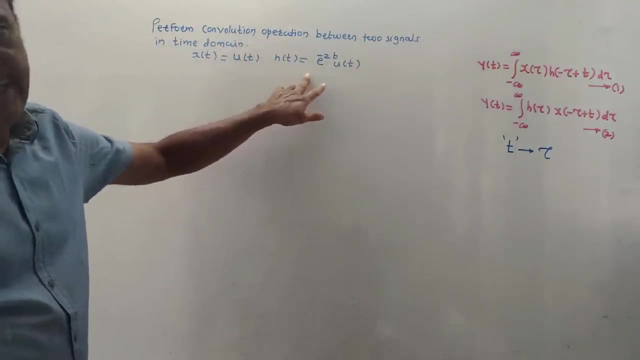 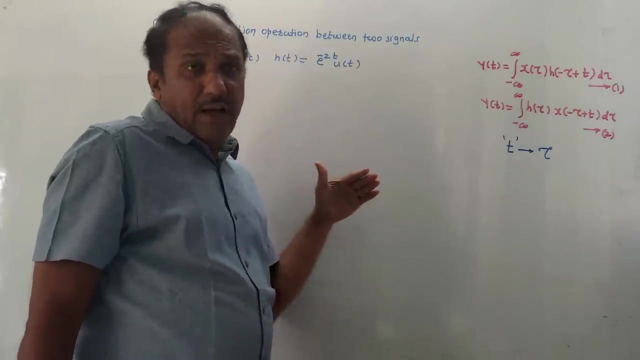 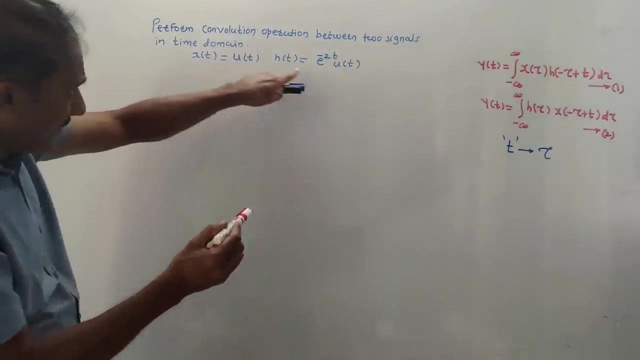 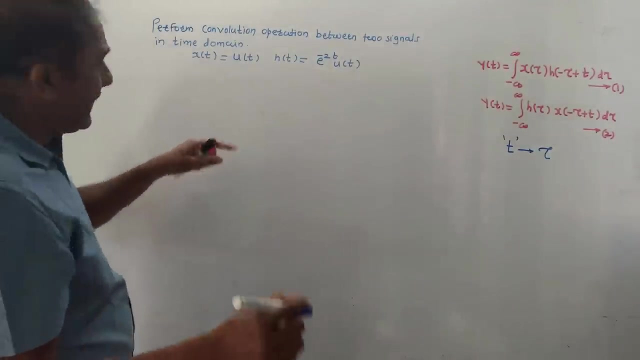 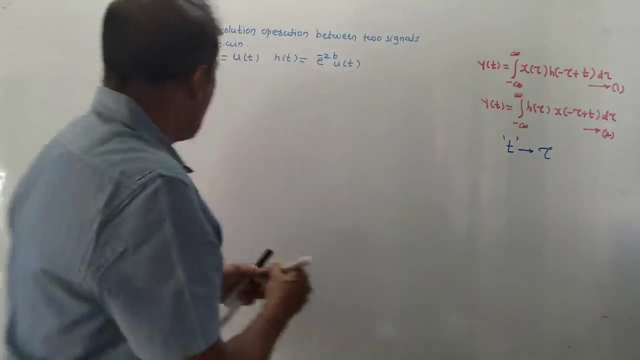 numericals. the problem is for convolution operation between two signals in time, domain x of t or h of t. given signals are there: a u of t, u of t means unit step uh before that. before starting it, so first step, i will simply replace every notation t by new notation tau. 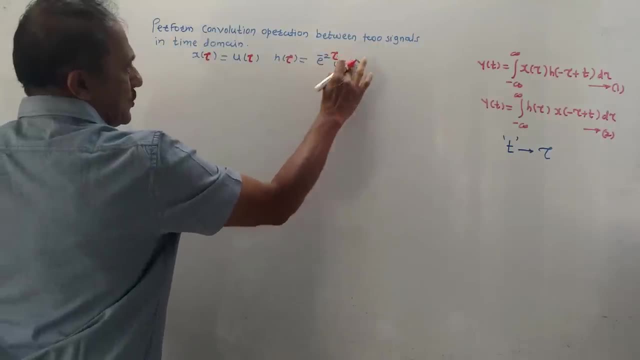 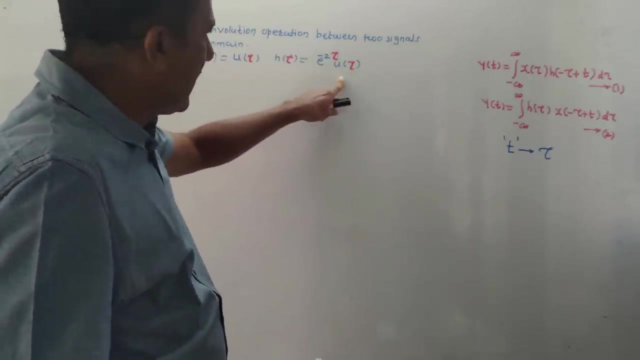 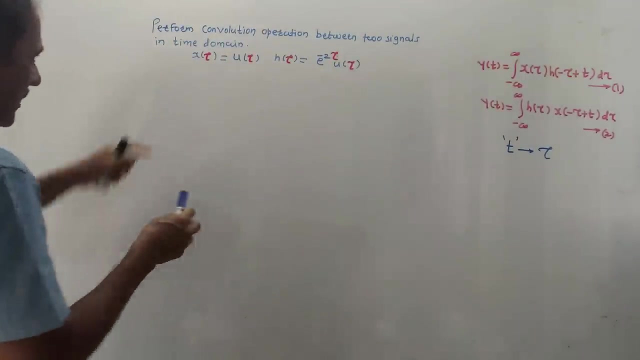 how may? just to give the indication key, we are performing the operation in different domain. i'm looking convolution: integral meaning remains same sip notation used, but no notation change. now see first signal is u of t and u of tau. that is a unit step. if i want to draw the diagram of unit step, 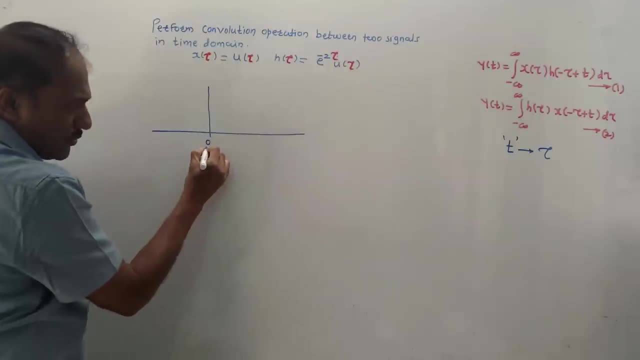 everyone knows here zero means t is equal to zero. now see, in normal case we write t here. this is convolution. so in place of t we have to do tau notation. now diagram of u of t is like this: from zero to infinity, its amplitude is one. this is the standard. 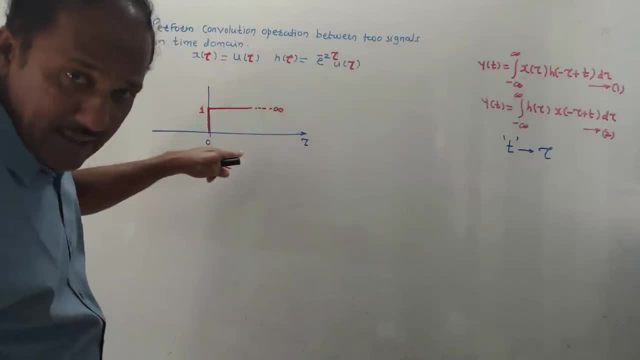 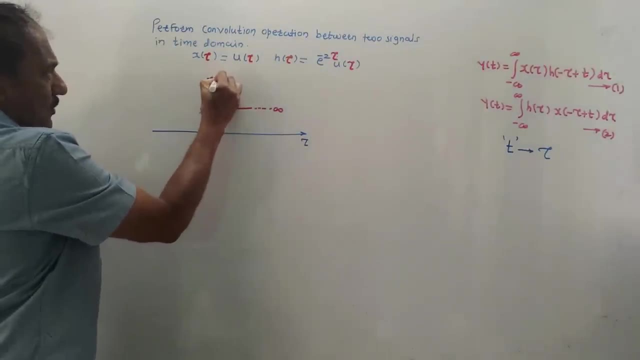 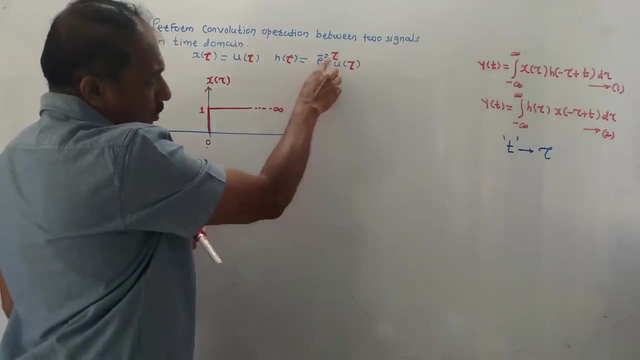 diagram. remember we are not giving diagram in the exam, we are giving only equation. you have to draw the diagram. i have drawn this diagram of x of tau signal, which is u of tau. that is unit step. second diagram i have to draw is e raise to minus two tau, u of tau. 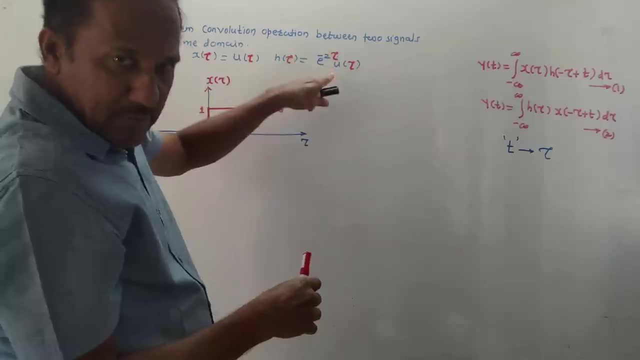 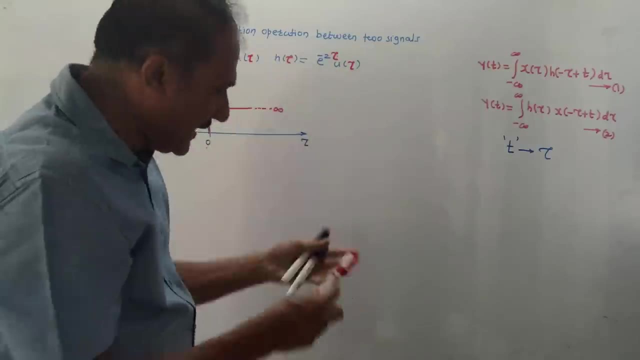 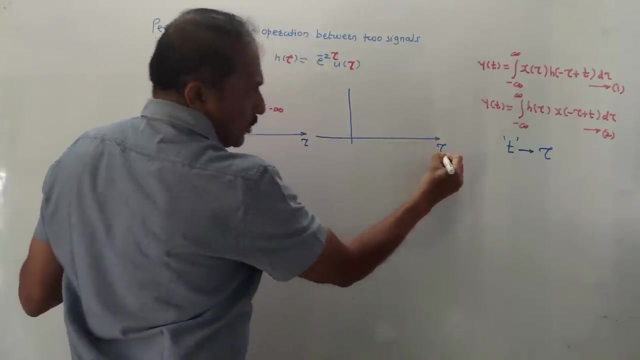 means e raise to minus two t u of t. as i have told you many times, that notation has changed. this means e is exponential, not minus, so exponentially decrease. so how to draw the diagram. on this axis we will write tau, where usually we write t. on this axis we will write h of tau. 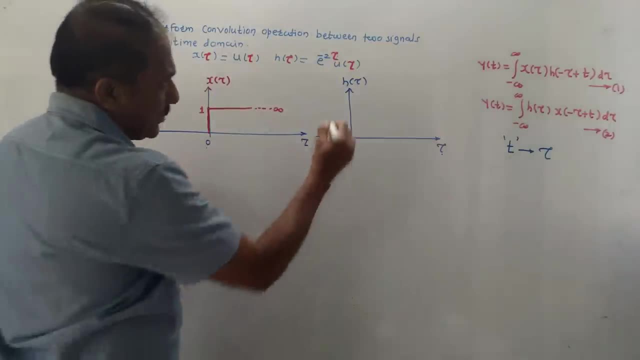 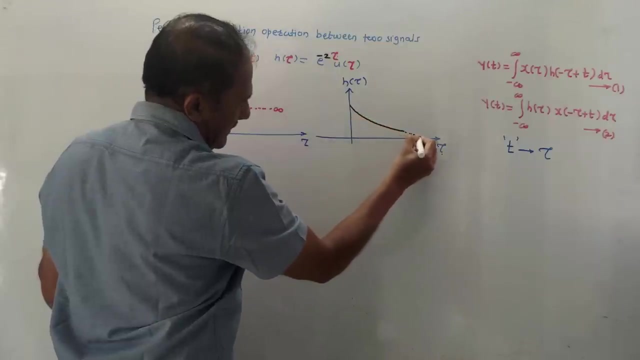 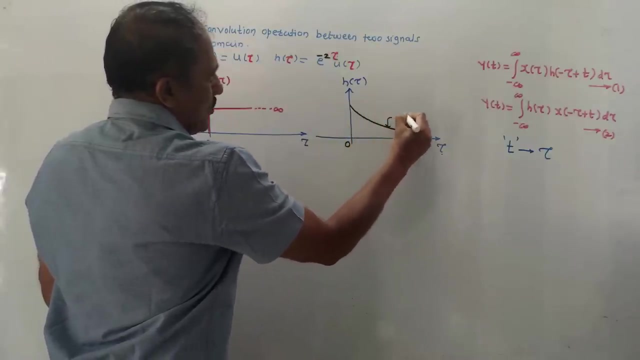 we will write second signal. now how to draw it. its exponential sign, minus sign, minus two tau. so it will exponentially decrease. like this: its like this, its zero. here we will write e raise to minus two tau. remember this concept i have told you in last video. if any value is multiplied by unit step, 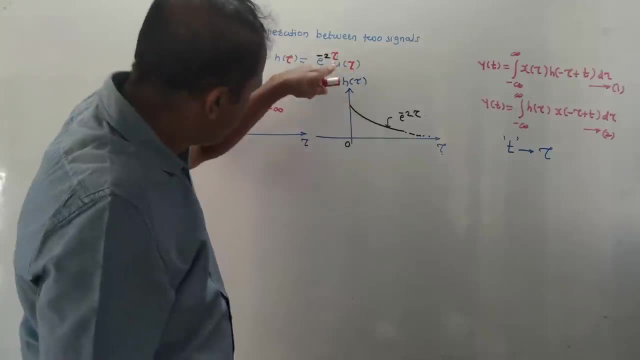 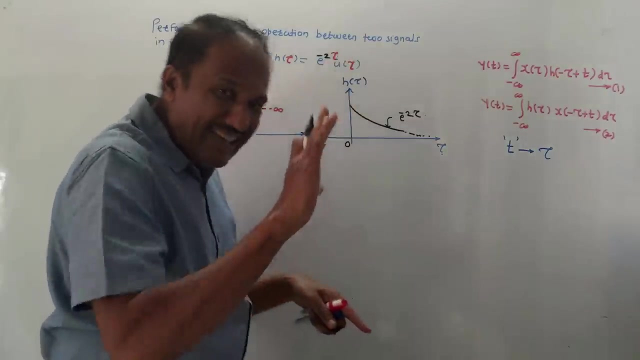 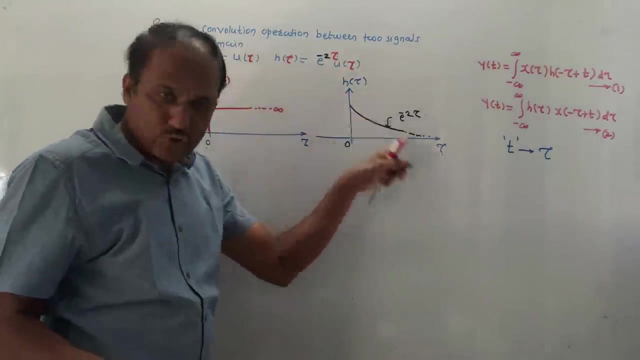 means u of tau and u of t. this means that signal is only on the positive side. there is no other significance after that. u of tau should not be used when drawing the diagram. that diagram e raise to minus two. tau should be drawn only on the positive side. 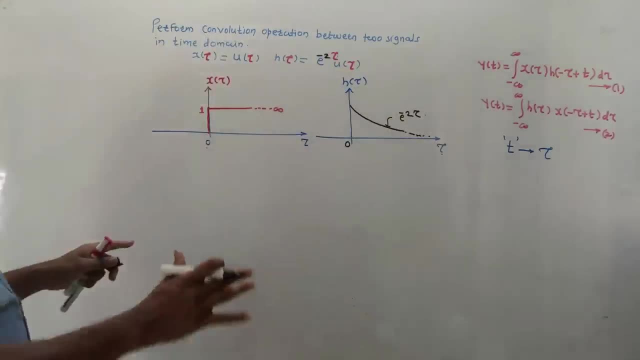 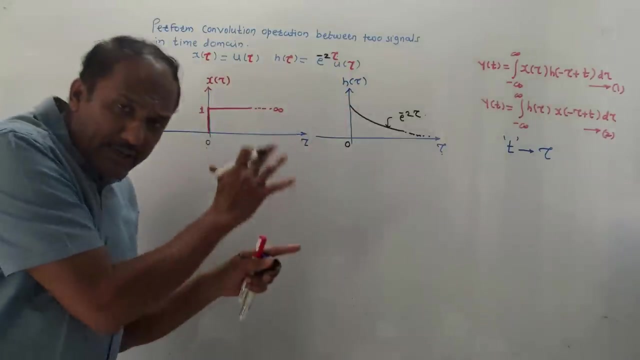 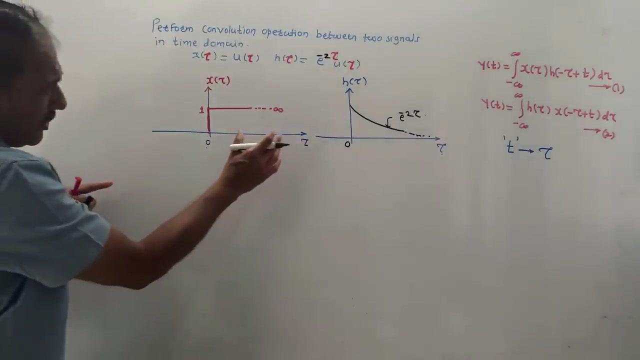 it will not come on the negative side. that is the only significance. now you have to think like this: one x and the other h. which signal should be folded means one signal should be kept as it is and the other should be folded and should be shifted. so its very simple. 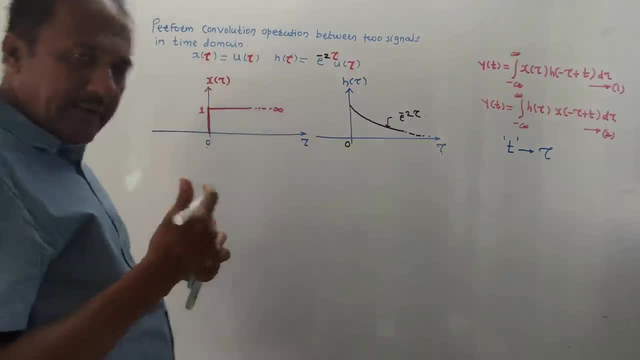 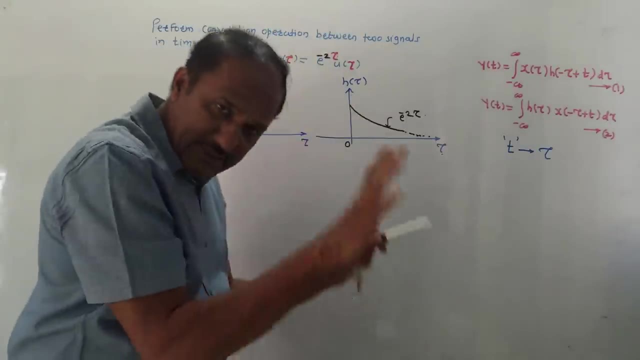 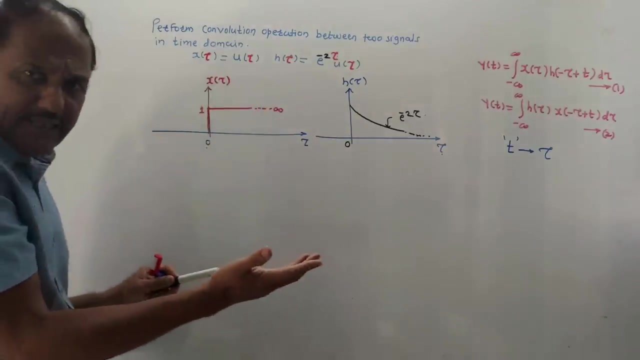 if i fold this signal, then it will be very simple. but if you do the opposite in the exam, it will not make any difference. it is not at all wrong. answer will remain same. but presently, if i fold this signal, then it will come on the negative side. 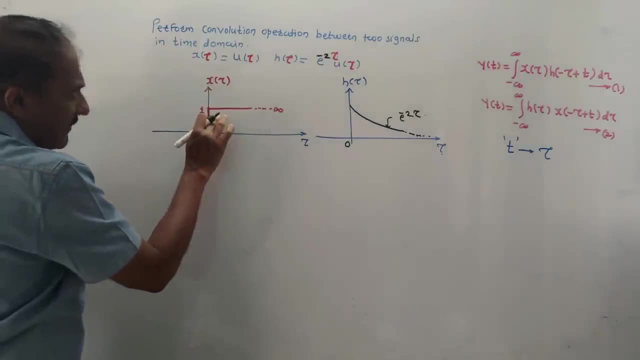 so it will be very simple after shifting. so i will draw the folded version of this diagram that is denoted by x of minus tau, as it is on the positive side. i will make a new diagram. the whole signal will come on the negative side, from minus infinity. 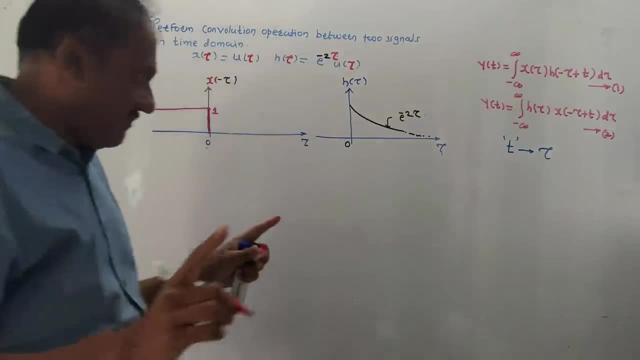 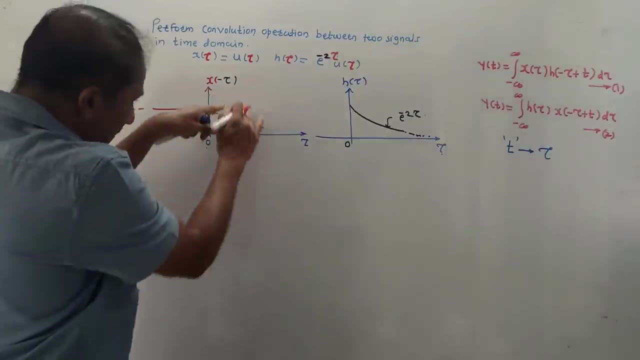 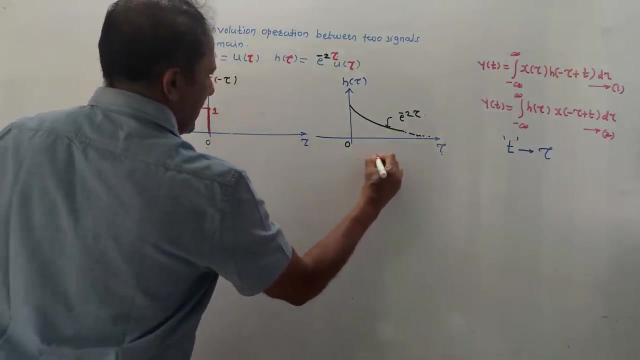 to zero, the amplitude will be one. now see, just to avoid confusion in the exam, the diagram which you will fold. you have to keep that. before this you have to delete the diagram. so give some numbers, say figure 1. i have given the number in the bracket. 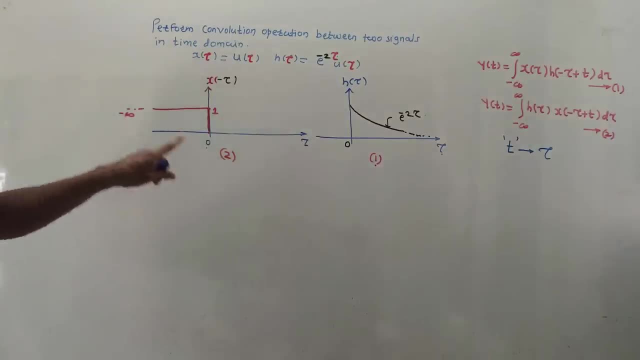 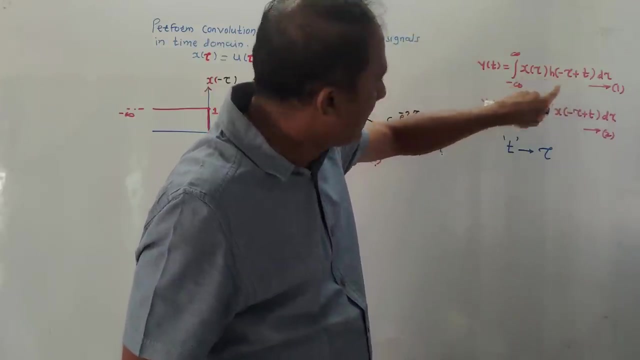 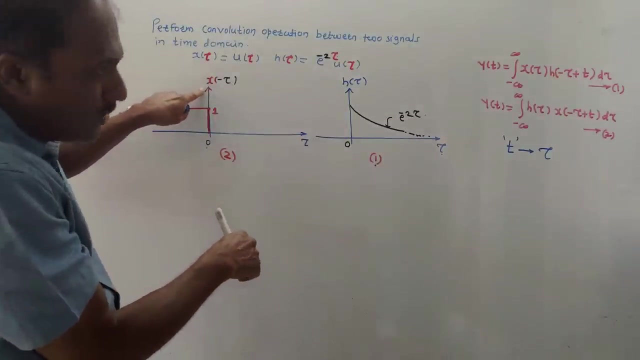 this is figure 2. figure 2 is the folded signal. you have to think like this. i have two formulas. in the first, formula h of minus tau, means h is folded. in the second, formula, x of minus tau, means x is folded. in this numerical, i am using folded version of x. 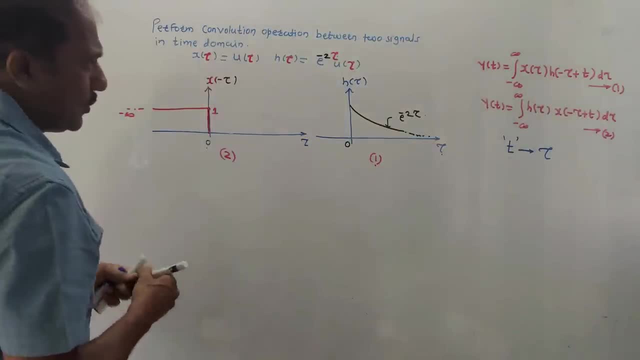 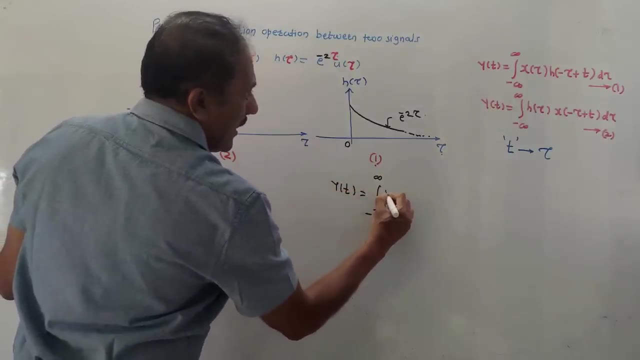 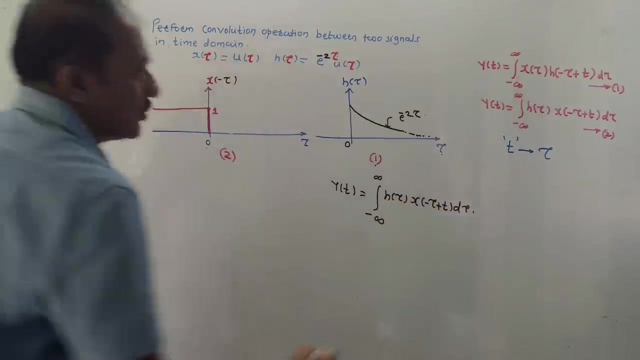 so i am making use of formula number 2. so let us write the formula number 2. it is: y of t, is equals to integration, minus infinity to plus infinity, h of tau, x of minus tau plus t tau. i have to use this formula now, most important part. 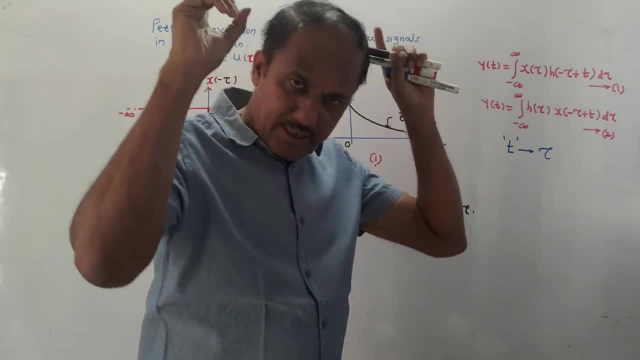 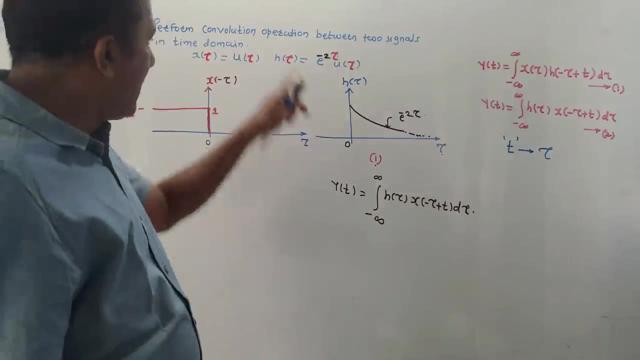 this is the beginning part in every numerical. we have to do this first step. what all we have to do? first, we have to draw one signal as it is. second, we have to fold it and write the formula of convolution integral. this means we have done tau notation. 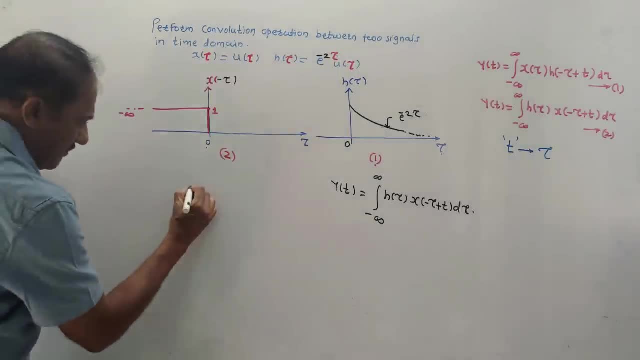 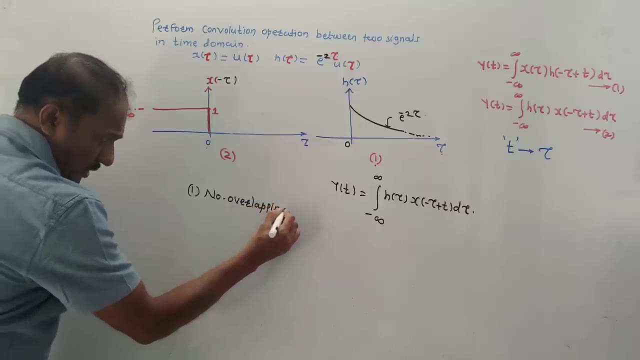 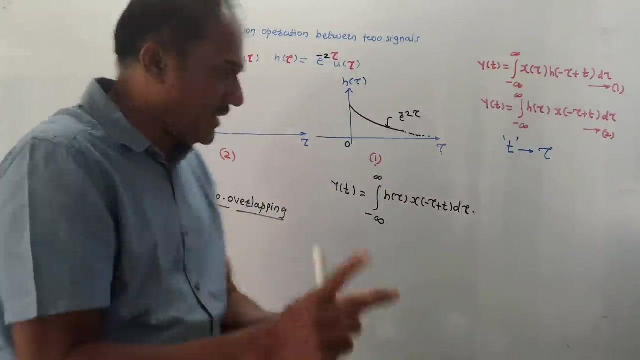 now i have to see three conditions. first condition: no overlapping. what does this mean? listen carefully. this is a little tough part. the folded diagram. i have to shift it. we have only two options: either i can shift this diagram to the left, or i can shift this diagram to the right. 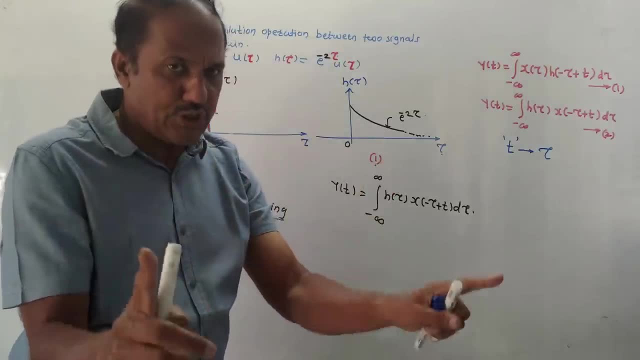 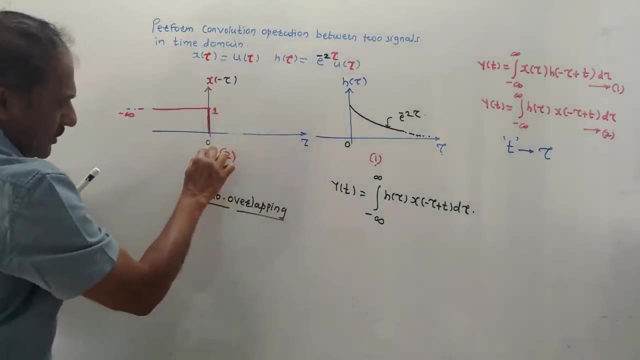 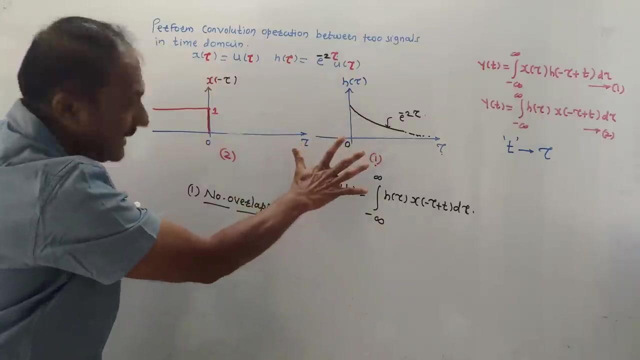 overlapping means common portion between two diagrams. think like this: if i shift this diagram to the right, like it is, till 0, i will shift it till 1, so it will come till 1. this diagram is in the positive side, so some overlapping will come. i want zero overlapping in the first condition. 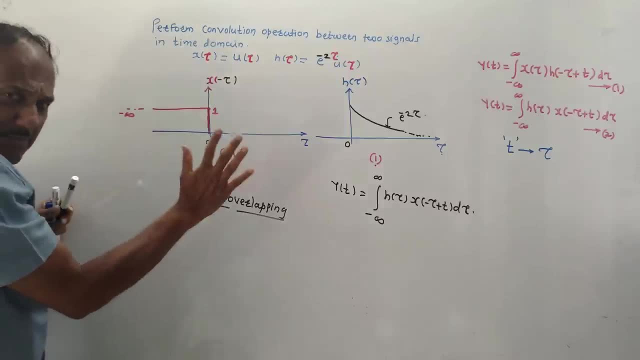 no overlapping. so i have to shift this diagram to the left with any amount. like if we shift from 1 to left, then this diagram will come till minus 1. so from minus infinity to minus 1 this diagram and this no overlapping, because this is in the negative side. 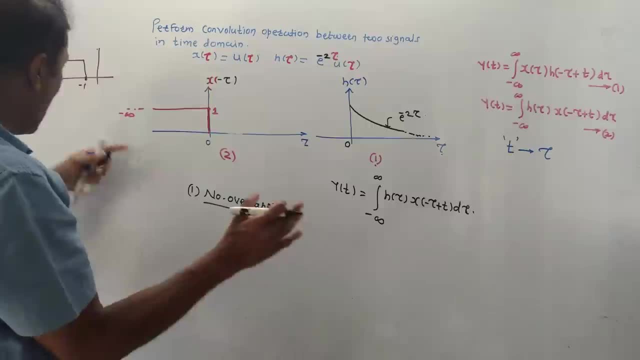 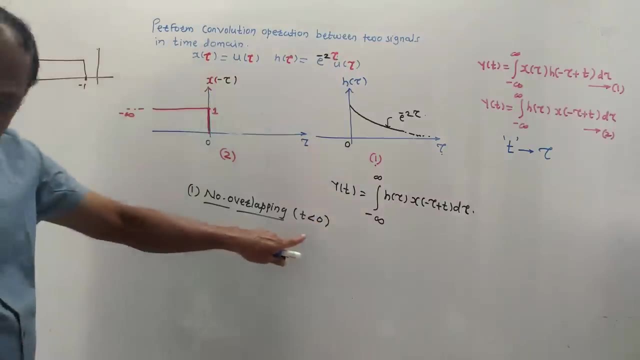 so from any amount, we have to shift it to the left. now, how did i tell you that we have to shift it to the left? we have to write the condition in the bracket t less than 0, because we have to shift it to the left. t is negative in the left side. 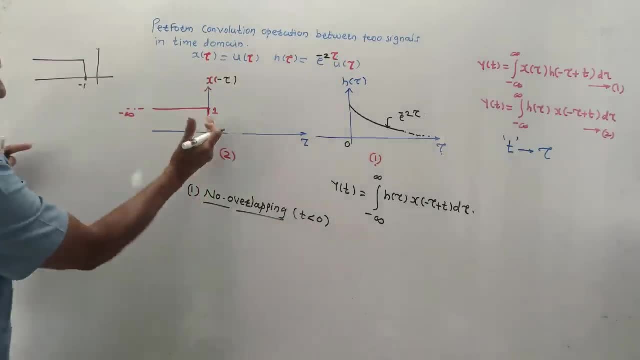 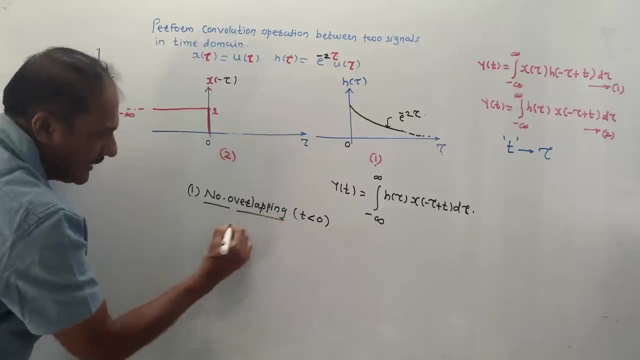 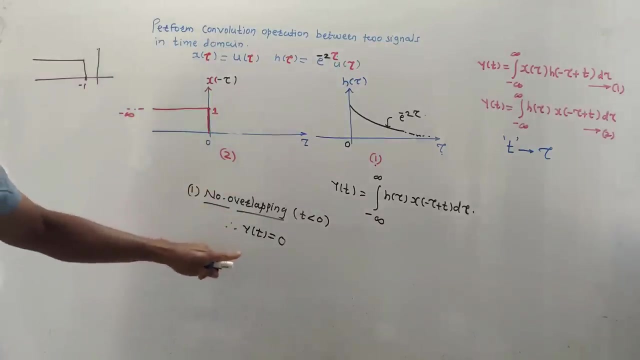 so i have written t less than 0. now in this there is no need to tell the diagram, it will shift to the left. there is no overlapping which i have already written. therefore, result of convolution y of t is equal to 0 in every numerical we have to satisfy. 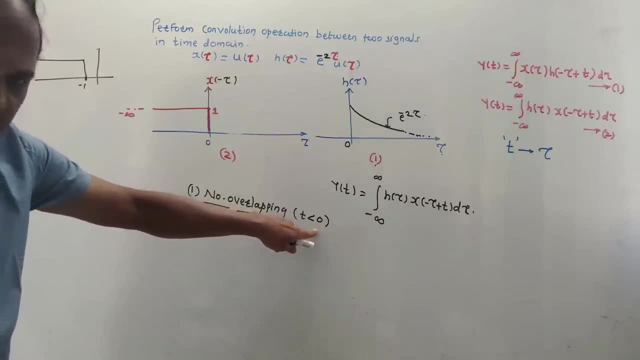 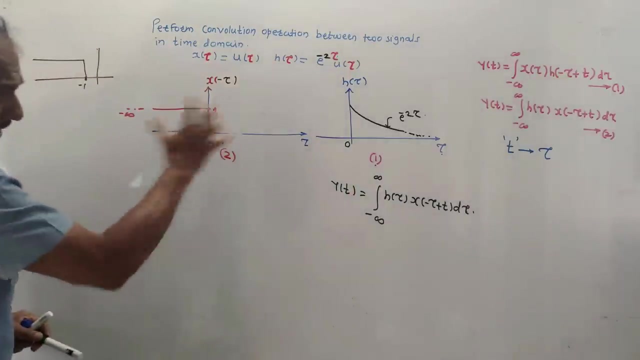 this first condition: no overlapping. t less than 0. this will shift to the left. so we have done t less than 0 and the answer of integration will be 0 because there is no overlapping. this is the first condition. second condition: now look, when can we have full overlapping? 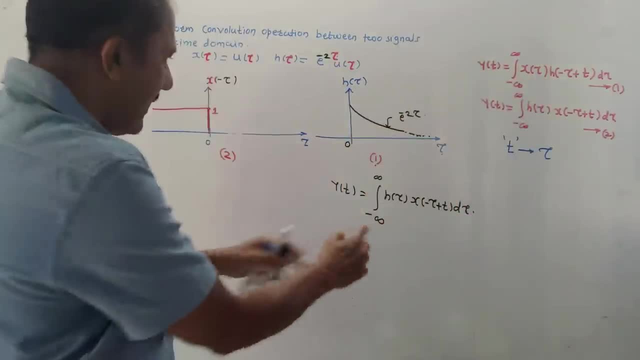 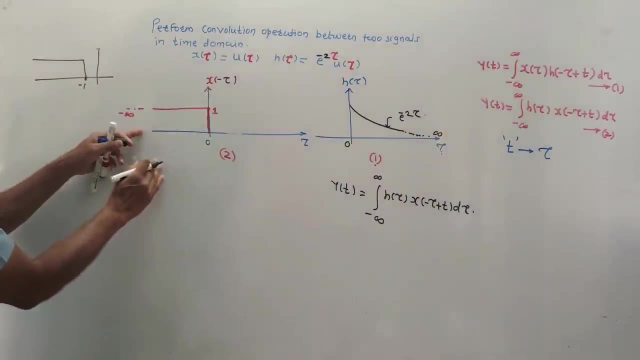 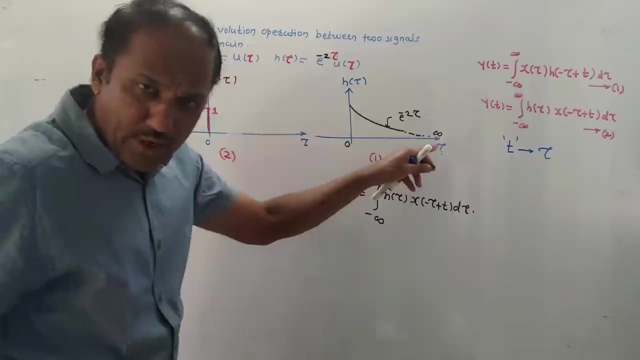 means when can we have full overlap of both the signals? one signal is this: from 0 to infinity, this is still infinity. if i shift this diagram, i will report this, this diagram from infinity, then only it will be full overlapping because this is minus infinity to 0. 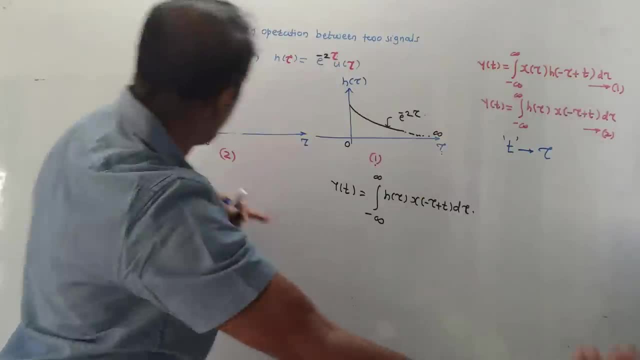 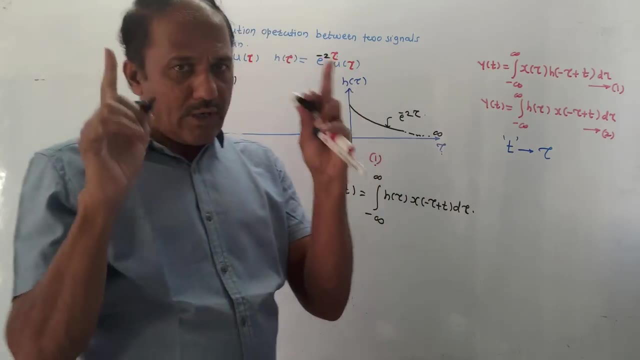 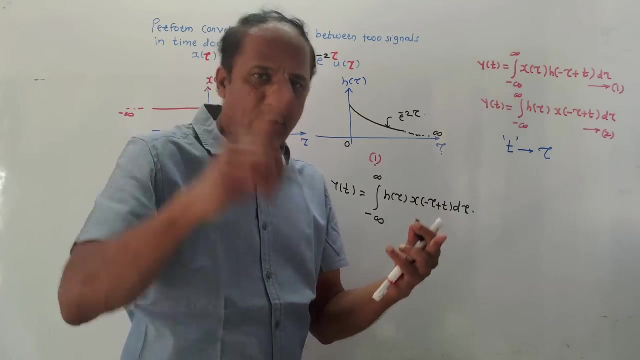 if i shift from infinity amount to the right, then this will be 0 to infinity and this also 0 to infinity. so this is full overlapping. now one very, very important thing: always: if, while doing full overlapping range is till infinity, means overlapping is till infinity, then that condition. 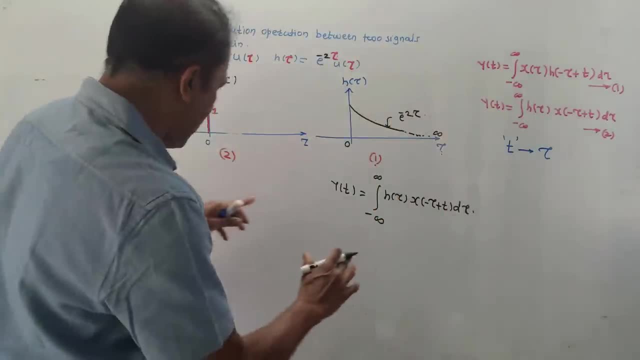 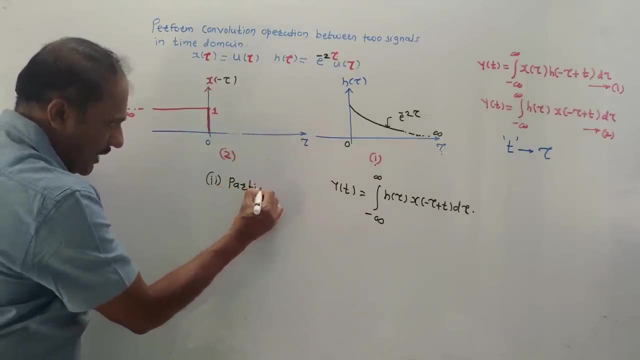 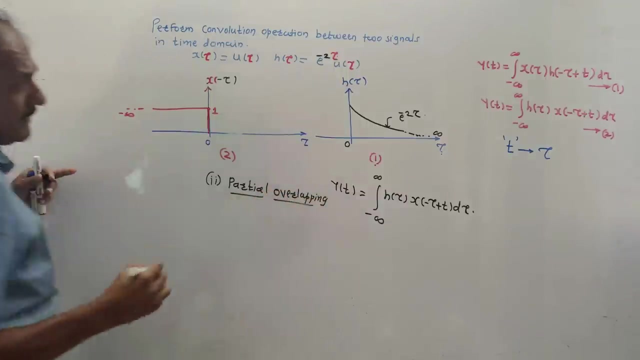 should not be used. so only we have one condition we have not used. only one condition is left, that is partial overlapping. so i am writing second condition: partial overlapping. what does this mean? we don't have to overlap the whole signal. there should be some partial overlap, like this diagram: 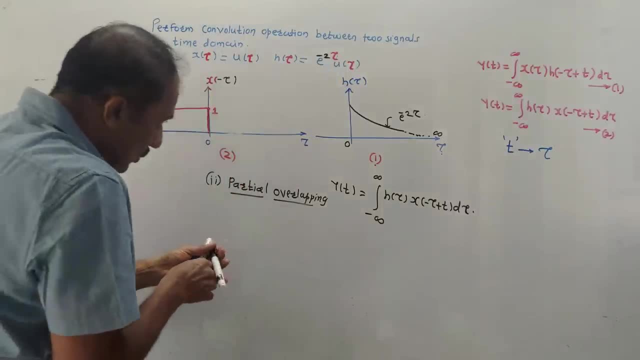 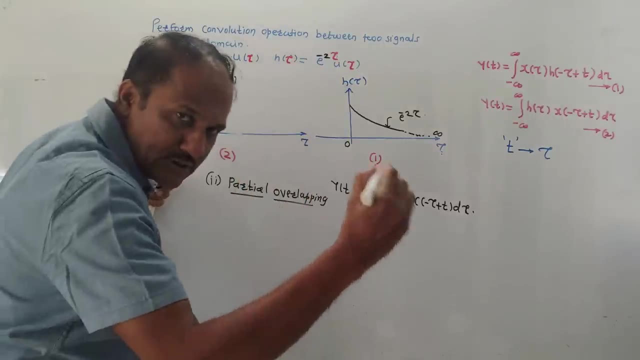 if i shift from one position to the right, then this diagram i have to shift from one position to the right. this diagram is minus infinity to 0. i have to shift it towards right by one position, so this will come till 1. this diagram will come like this: 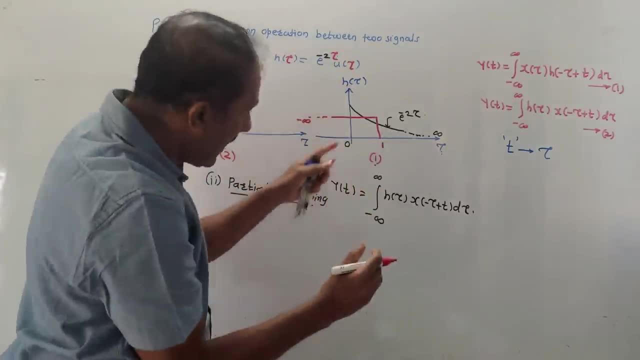 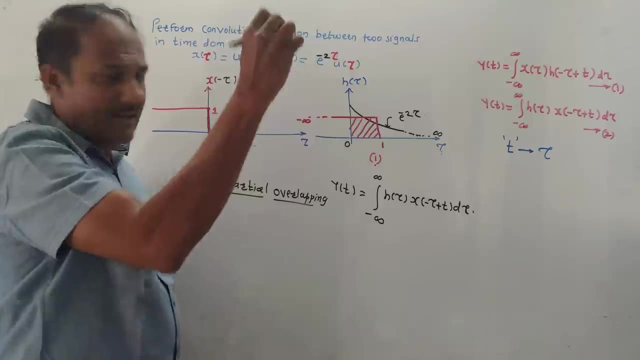 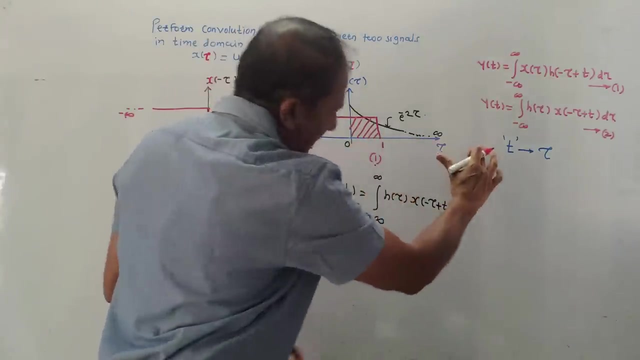 and this will be minus infinity, as it is from minus infinity till 1. now observe what will be the common portion. this is the common portion, this is the overlapping, but this number 1,2, if i shift from 1 to 2 then it will be 0 to 2 overlapping. 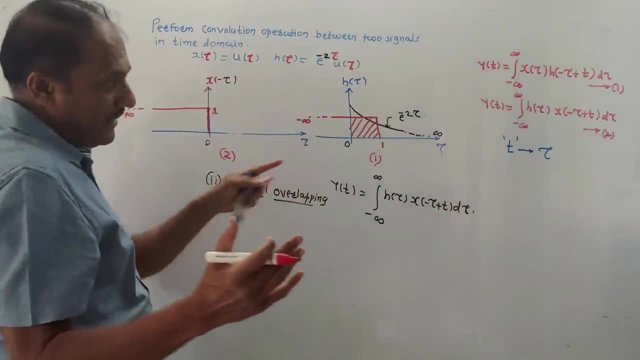 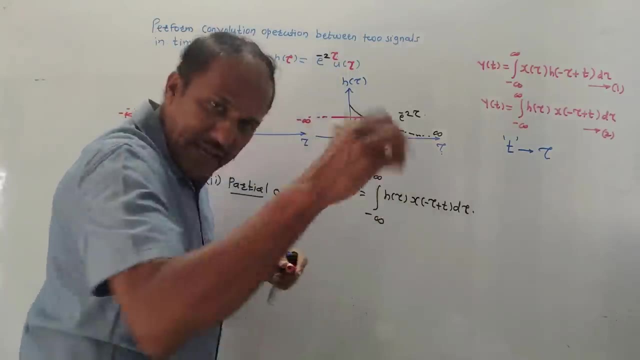 if i shift from 2 to 3 then it will be 0 to 3 overlapping in exam. you don't have to write like this: 1,2,3 means you can take any amount, so you have to write like this: here you have to write t. 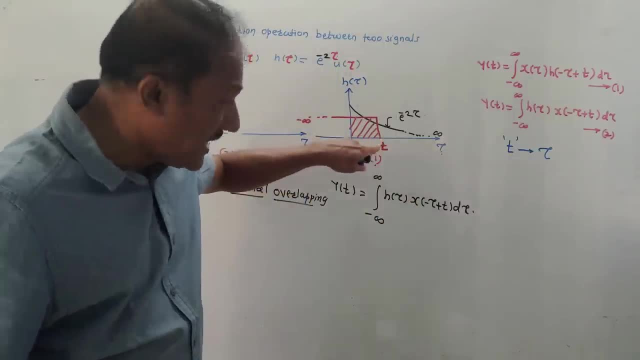 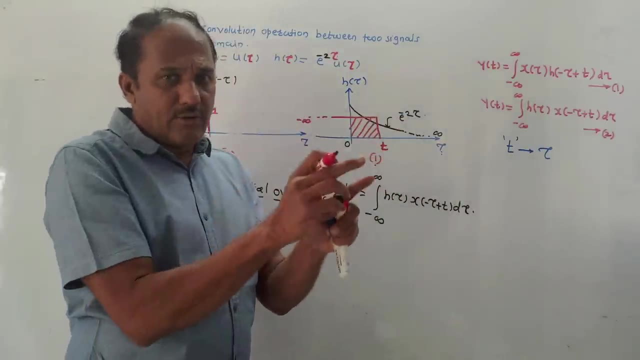 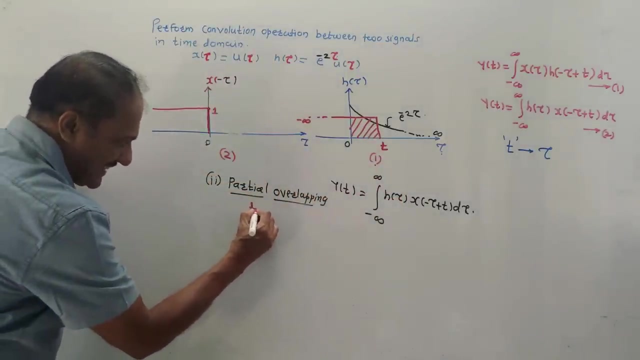 where t can be anything. keep in mind, if t is any fixed number which we will put value like 1,2,3. so, like i told you, t is equal to 1,2,3. you don't have to write like this. you have to write in notation terms. 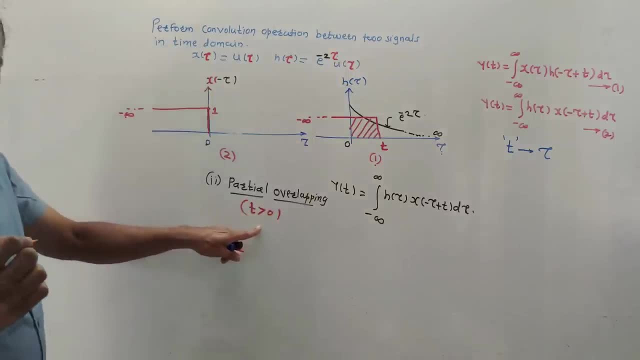 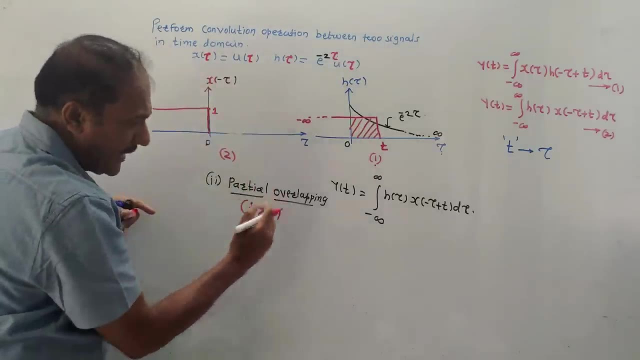 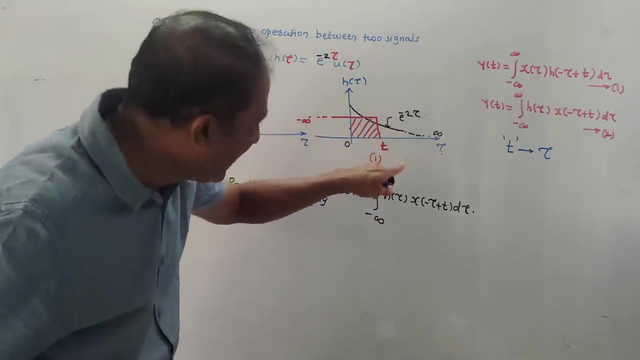 so, for partial overlapping, i will write the condition t greater than 0, from where this condition came. how is this written? very simple technique. i told this diagram: if i shift from right, this diagram, towards right, by t position where value of t is not known, as i told you. 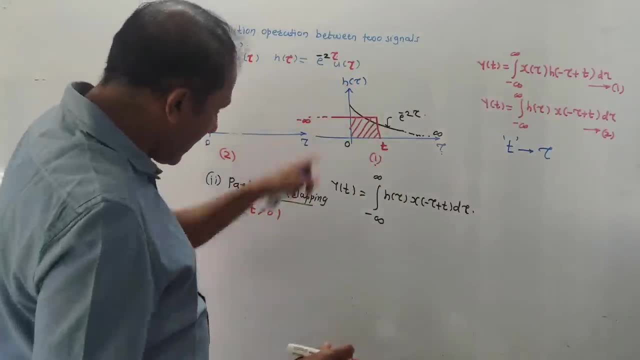 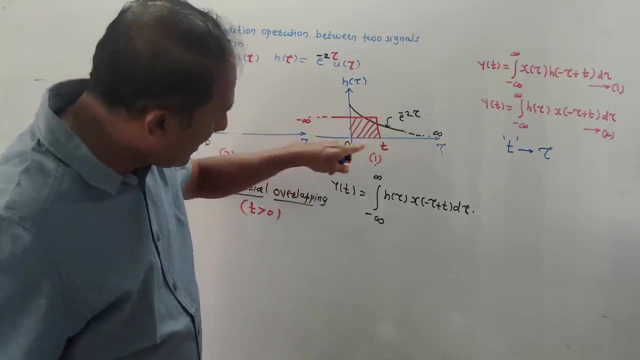 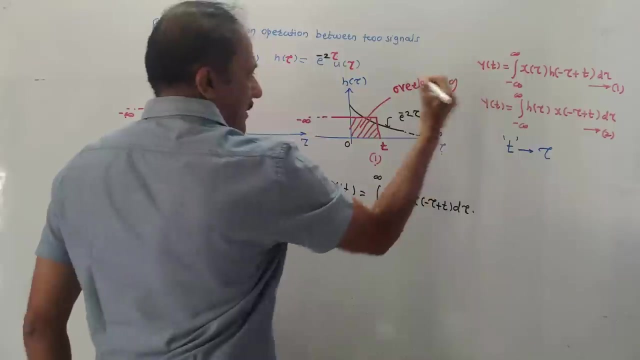 you have to write in notation terms. now one more important thing, as i have made this diagram, you have to always make combined diagram in one diagram. you have to show both signals and this overlapping. this is the overlapping. this is compulsory. you have to show this. now the remaining part. 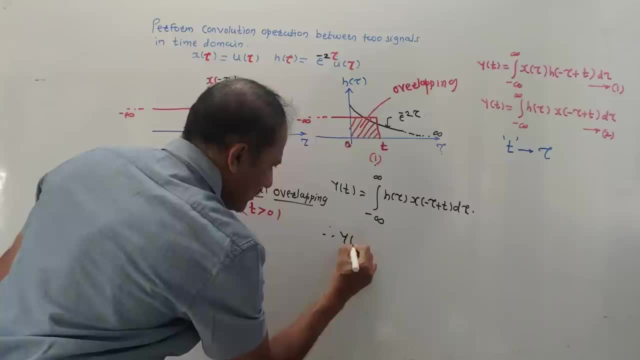 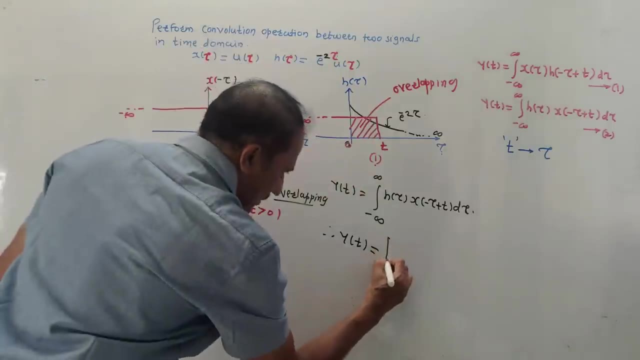 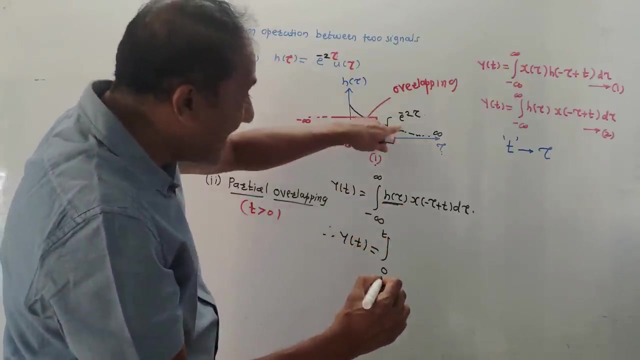 is very simple. this is the formula. let us put the values in the formula. now see this is general integration. from where to where is overlapping from 0 to t. so limits of integration will be 0 to t. see in formula h of tau. h of tau means. 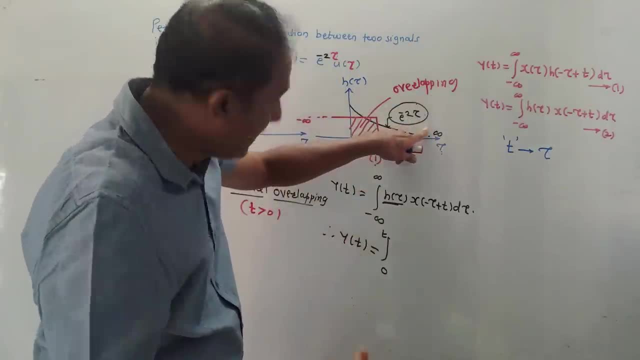 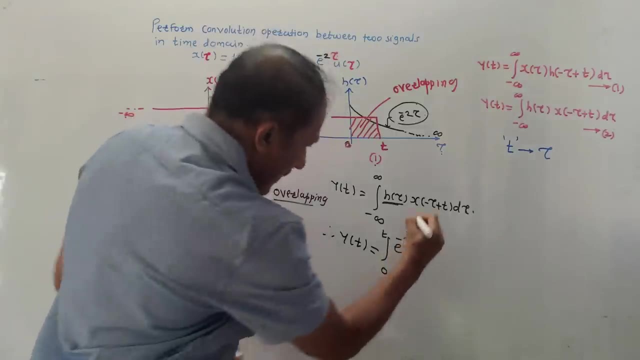 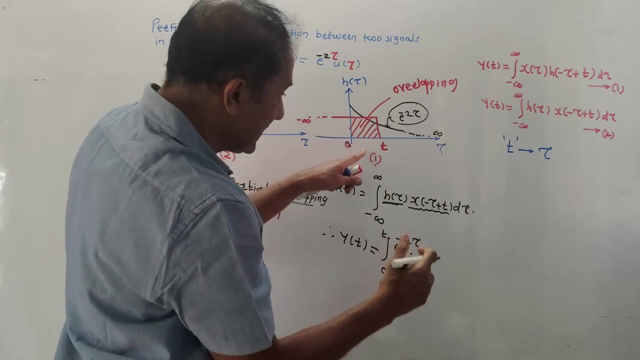 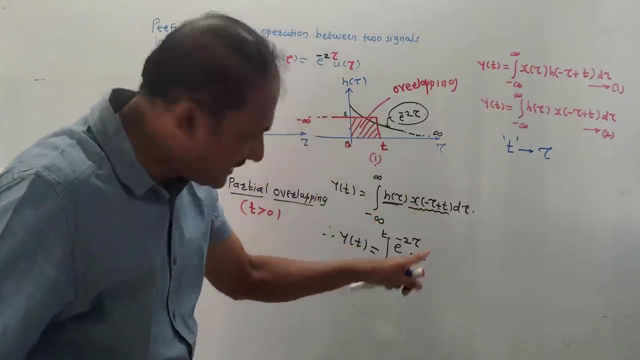 its value. how much is the value e raise to minus 2 tau? original value is e raise to minus 2 tau. into this signal x of minus tau plus t. this means this folded and shifted signal. its value is to be written. value means amplitude. its amplitude is 1. 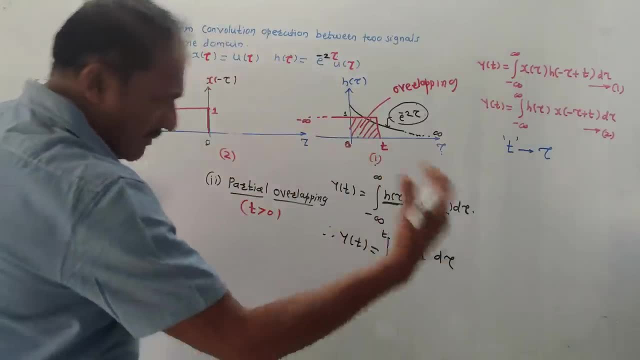 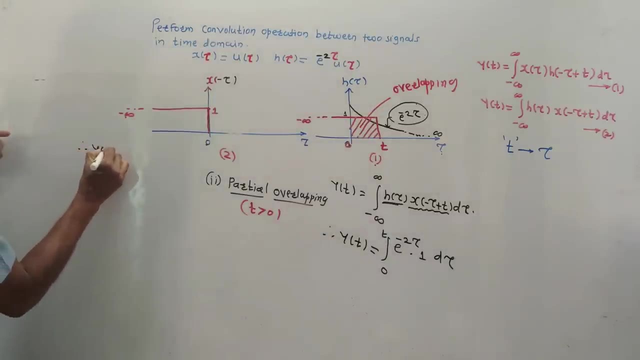 so i will write: 1. this is notation. instead of this we have to put values d, tau. now we have to solve this. integration is equal to in any integration. if in e raise to term, e raise to minus 2 t, as it is written, e raise to minus 2 tau. 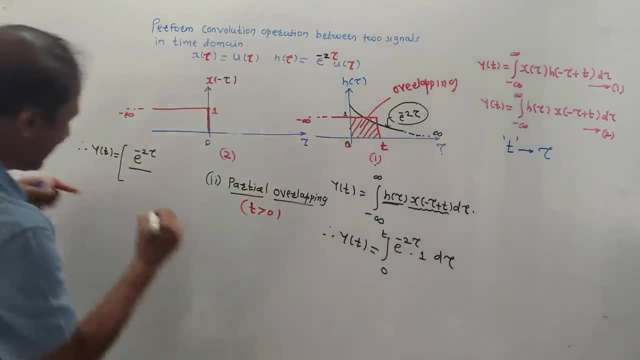 we have to divide. integration is with tau, with respect to tau, so whatever is other than tau with sign. we have to divide means minus 2, limits will be, as it is simple trick, i told. now put the limits first. we have to put limits instead of tau. 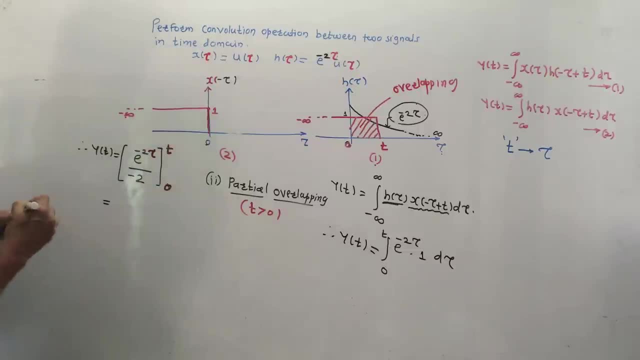 this is tau. we will put upper limit after that lower limit, so you will get e raise to minus 2, t minus lower limit e raise to 0. if we put 0 instead of tau, e raise to minus 2 into 0 means e raise to 0 will be. 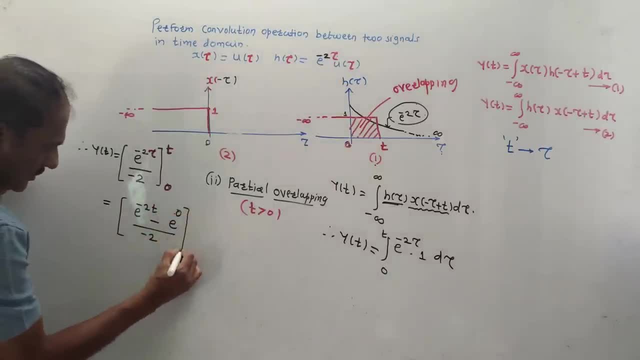 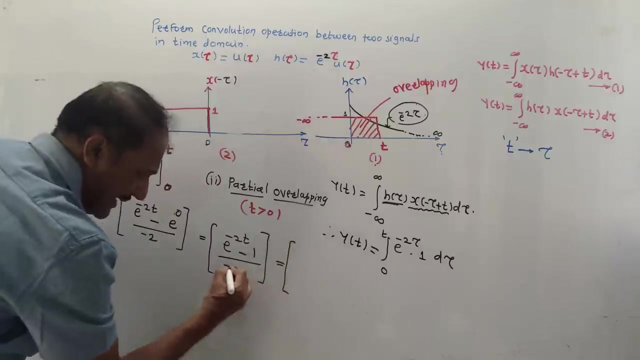 minus 0 plus 0 divided by minus 2. now simplify it like this: this is e raise to minus 2, t minus e raise to 0 means 1 upon minus 2. last step is sufficient. if you want to write more, you can write like this: 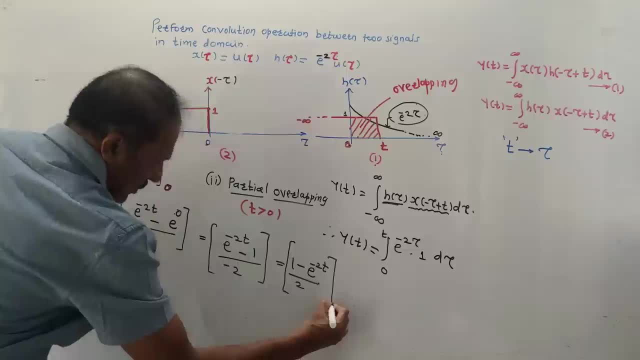 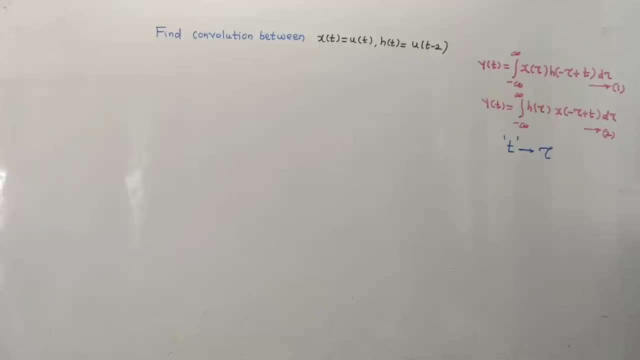 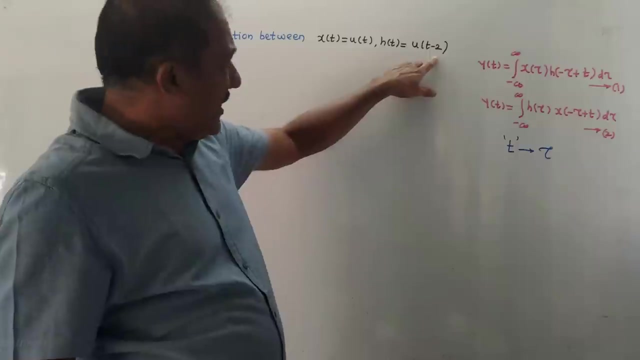 so i will write it like this: e raise to minus 2, t upon 2. so this is the answer of convolution for these two signals. next problem is convolution between x of t is u of t, h of t is u of t minus 2. this video may be a little lengthy. 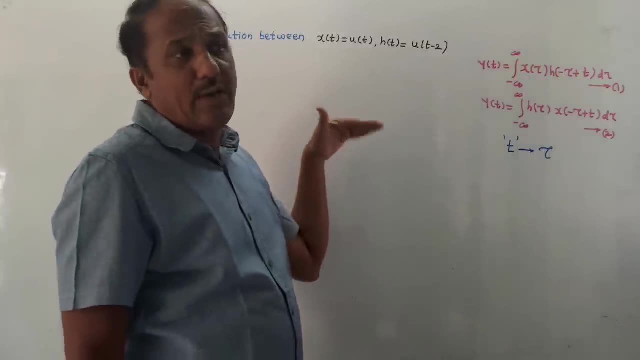 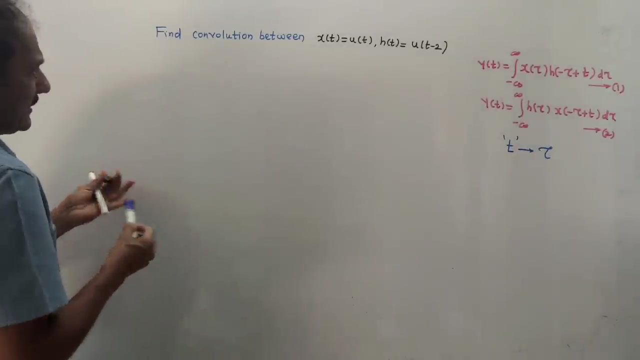 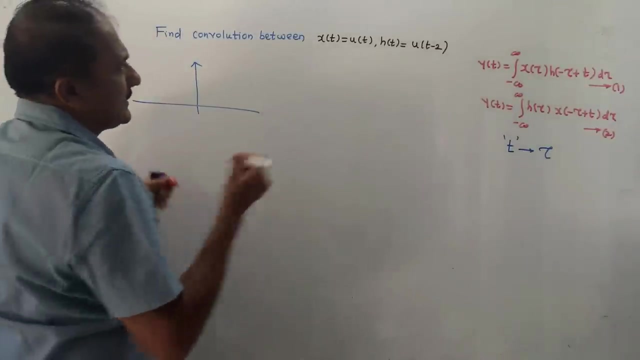 because i have to cover everything and it is not possible in such a short time. so i hope you can understand. two signals are given as usual. first we will draw u of t diagram, like we did in last sum. one signal is x of t before this, like the last sum. 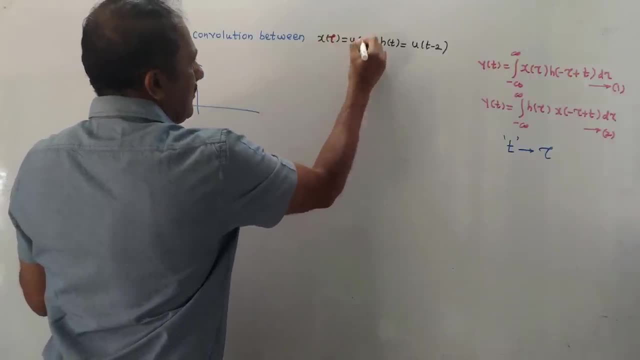 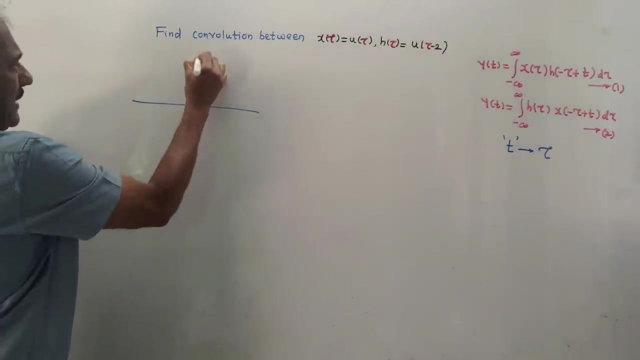 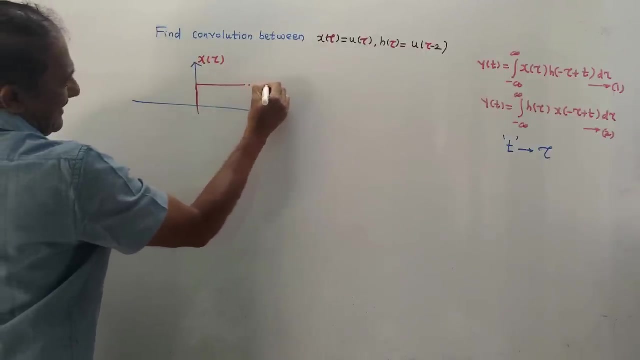 let us change the variables. we will use tau instead of t. this is a fixed step in every numerical. always change the variables. now. first diagram x of tau. that is u of tau means unit step. this diagram will be like this: second diagram: u of t minus 2. 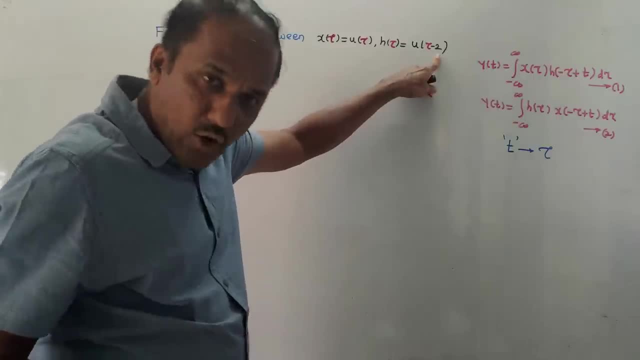 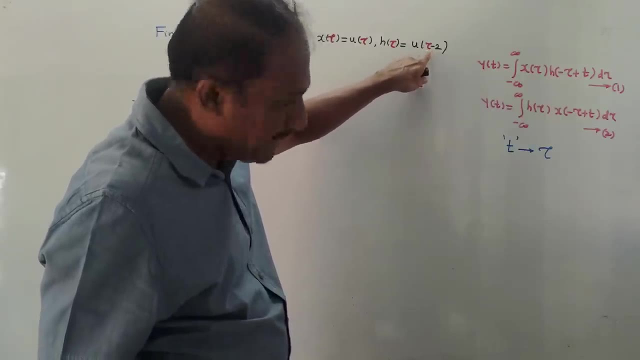 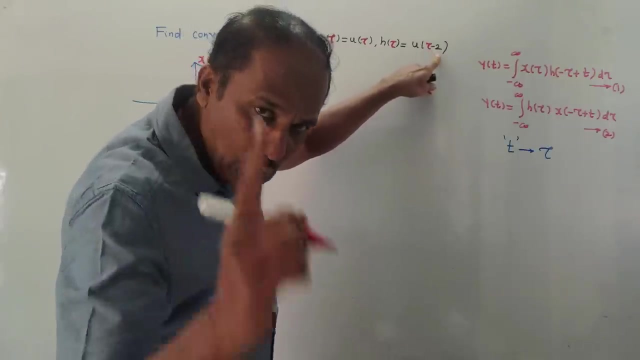 means u of tau minus 2. now we have already learnt the operation. recall the things. see the sign of bracket. if bracket has plus tau and minus 2, plus minus sign means it is opposite sign. so we have to shift right by amount 2. at that time we don't have to consider sign. 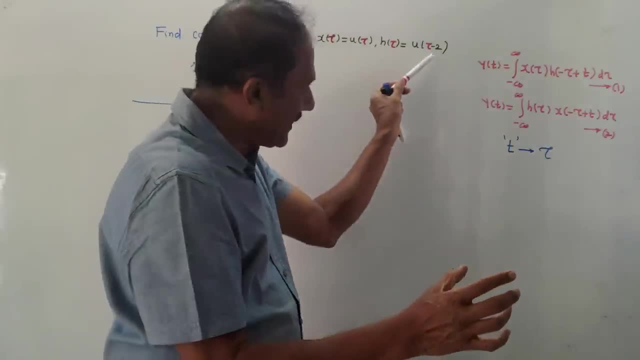 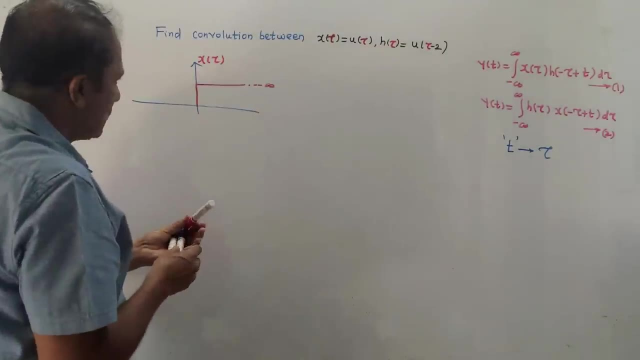 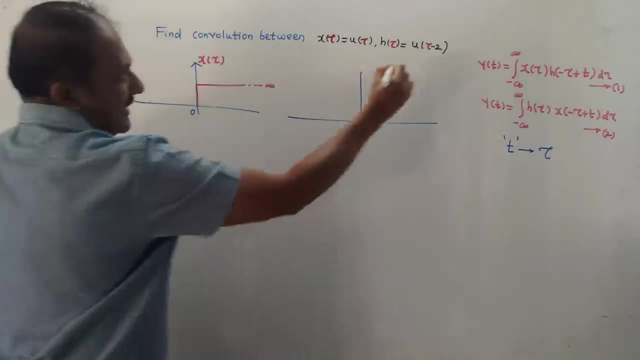 why we have to consider sign, whether you need to shift diagram towards left and right. if it is plus minus sign, then right shift by amount 2. so if i have to draw new diagram for h, then this diagram, u of t diagram, starts from 0, but u of t is minus 2. 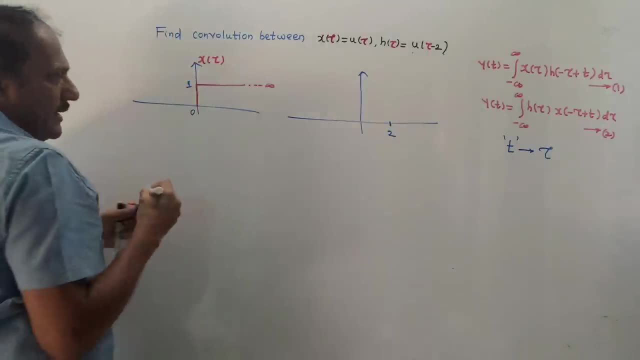 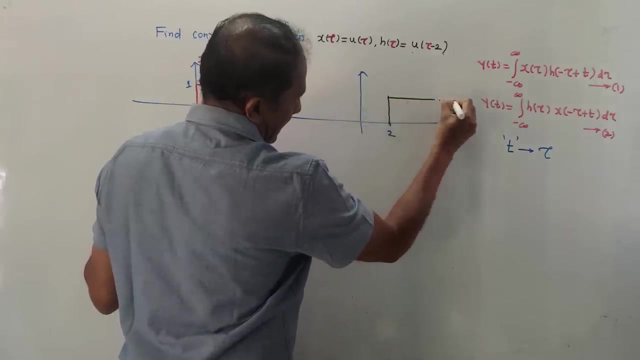 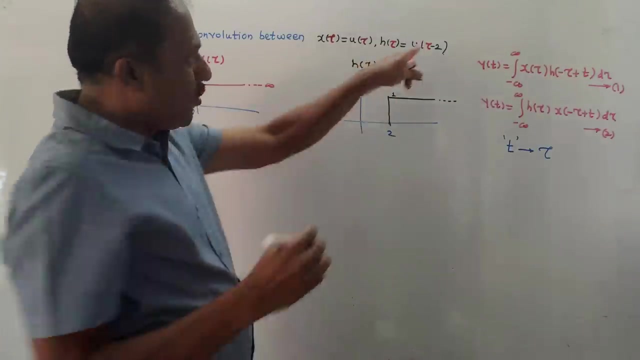 so it will start from 2. here also, amplitude is 1. only starting point will be changed and this sequence will be like this: this diagram will be like this: its amplitude is 1. this is the diagram of h of tau, that is, u of tau minus 2. 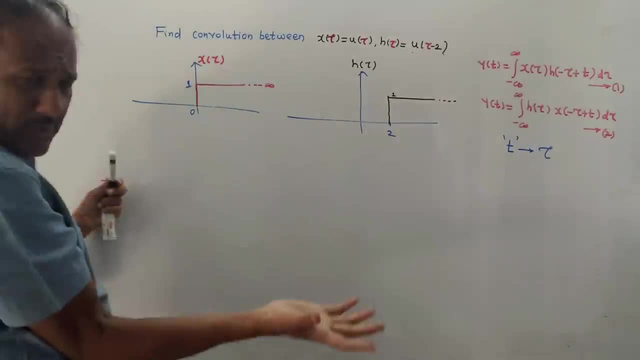 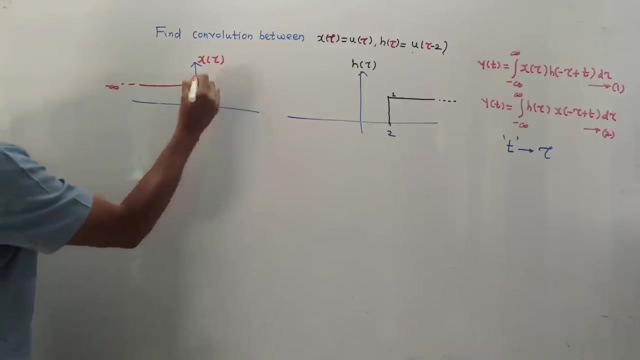 now think like this: from both. you can fold any sign. if you fold this, then it will be more easy. so lets draw its folded version. so folded version will be in left side. here is amplitude 1. here i write x of minus tau, as i told you. 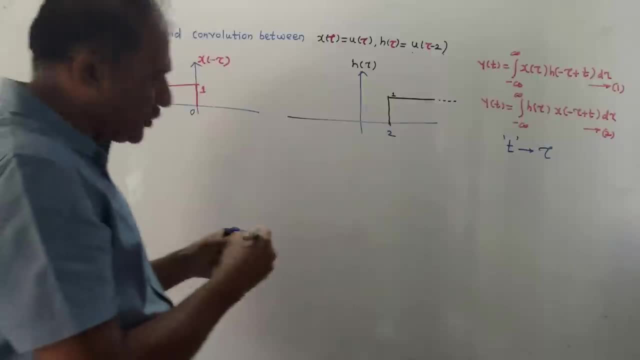 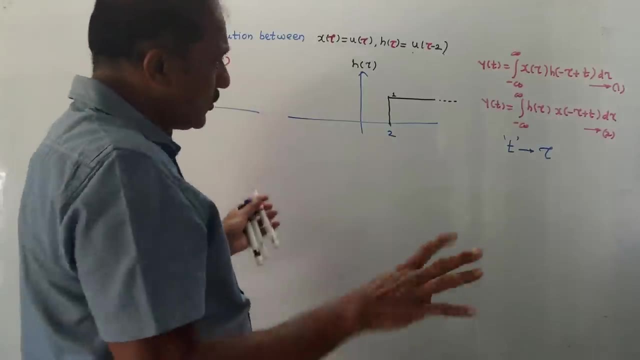 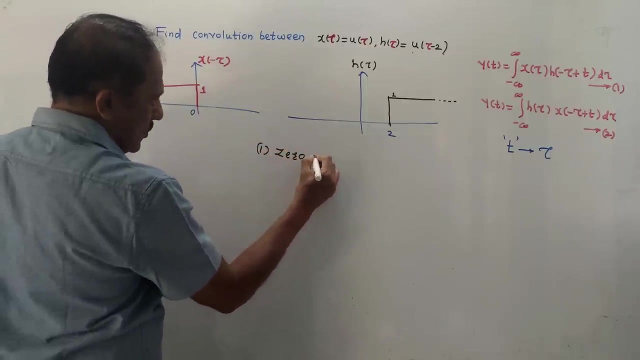 once you draw the folding sign. after that the original sign means x of tau. we have to delete it so that there is no confusion. now we have to use same logic which we used in last sum. first condition is 0 overlapping: 0 overlapping and no overlapping. 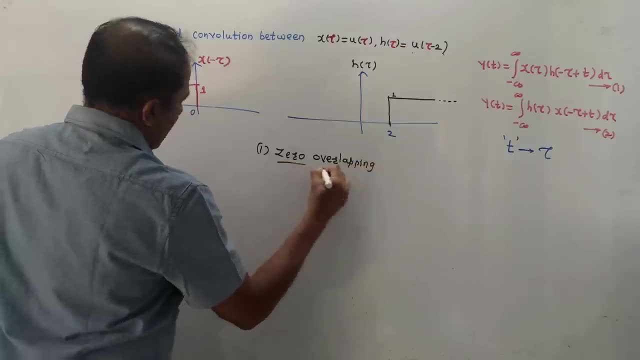 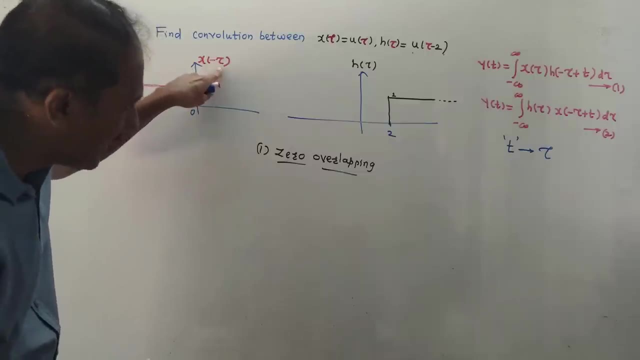 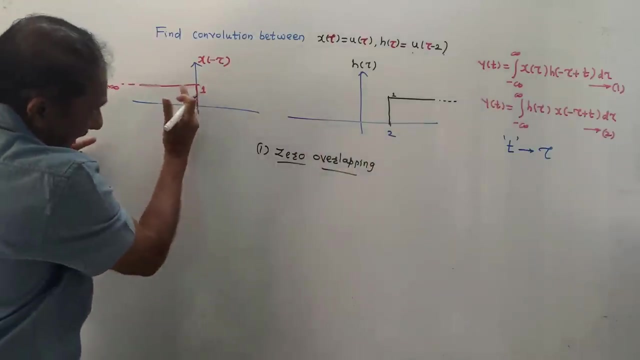 now observe both the diagram, this diagram. if i don't shift, which diagram we have to shift, always, always we have to shift the folded sign. if i don't shift, then also it is not overlapping, and if i shift right, like this. i will just explain the concept. 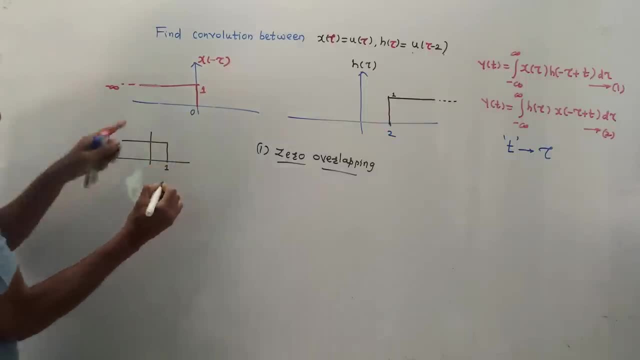 this diagram: if i shift right from 1 position then it will come to 1, but this diagram starts from 2, then also it is not overlapping. now, as you can see, i will shift till 1.9. this is starting from 2. still it is not overlapping. 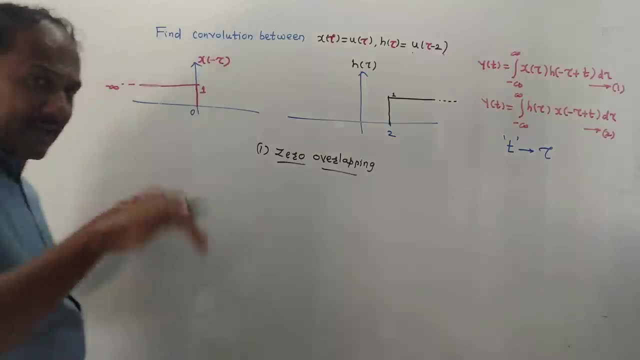 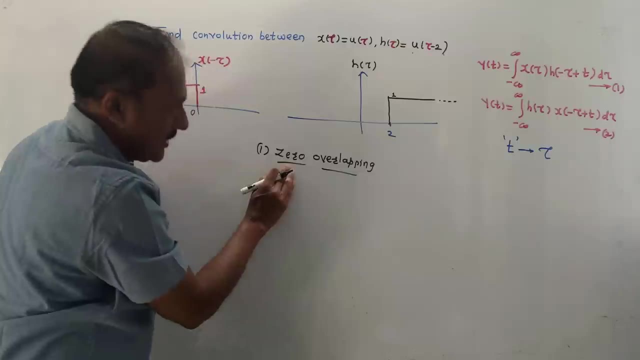 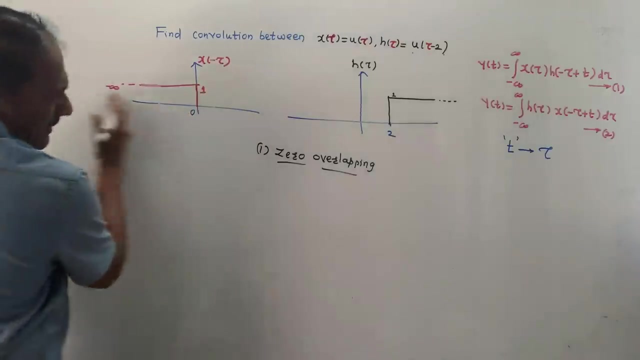 what this means is if you want overlapping. if you want overlapping, then you have to shift with more than 2 amount, but in this condition, i want 0 overlapping, like the previous sum. make it more simple. always remember this diagram so that you don't have overlapping. 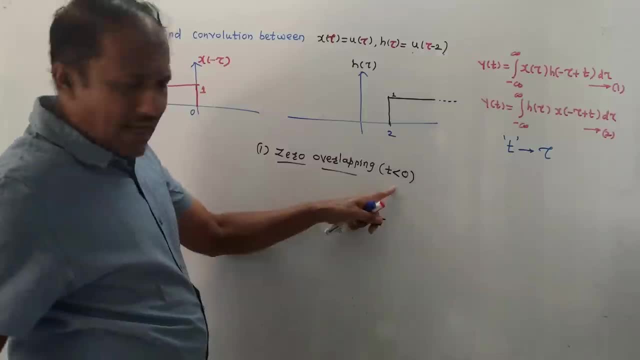 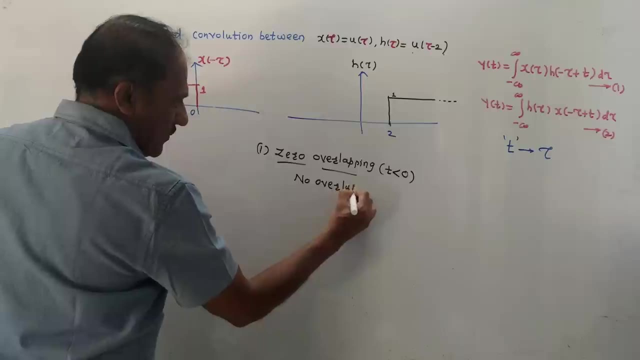 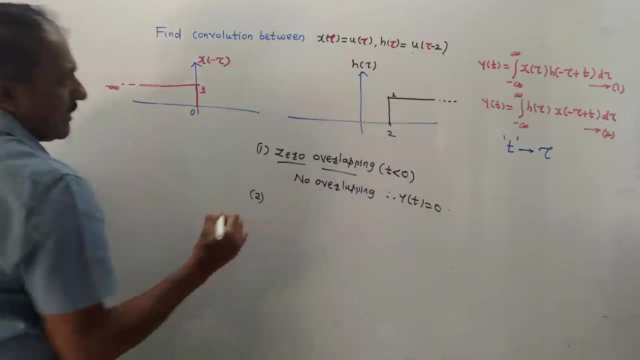 this is a very simple trick. i am telling you. remember this: t less than 0, no overlapping, and answer of integration will be 0. therefore y of t is equal to 0. second condition: partial overlapping. like the previous case, this diagram is from 0 to infinity. 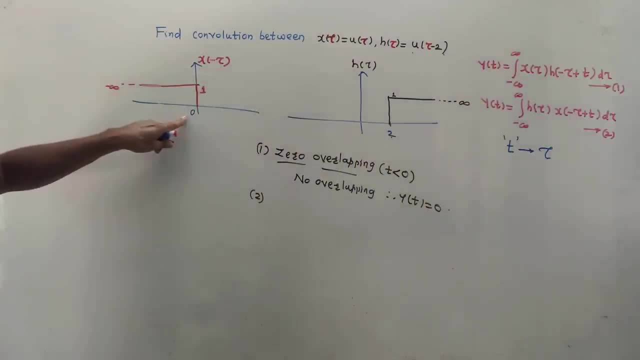 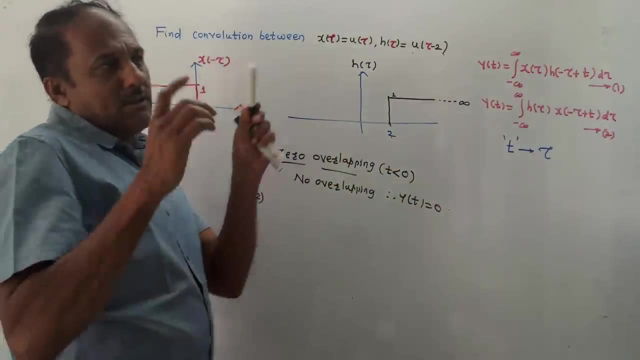 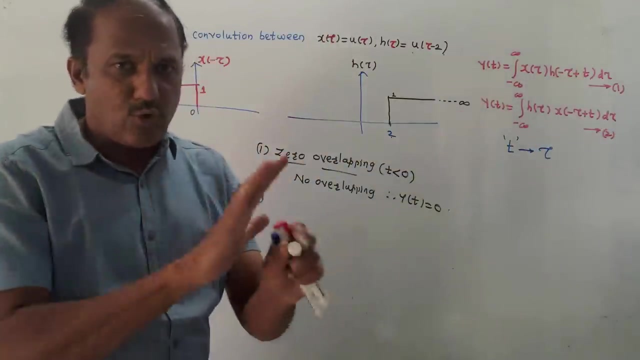 simple trick. this is from minus infinity to 0. if i shift it from 0 to infinity, then only it will be full overlapping. i have told you in last lesson, when overlapping is till infinity you don't have to consider that condition. that means we will not be considering. 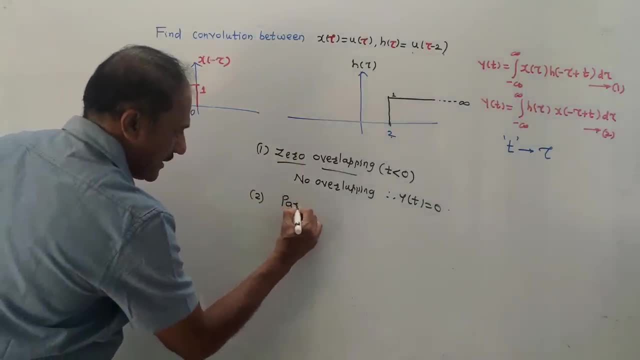 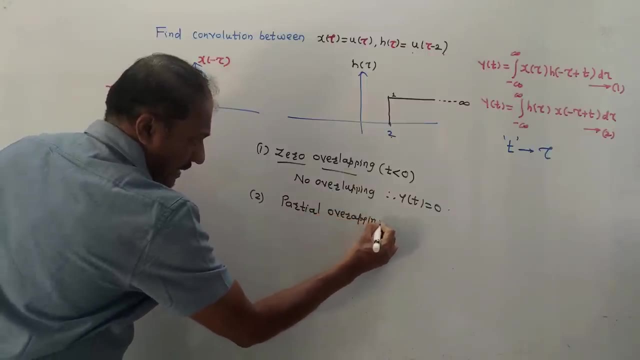 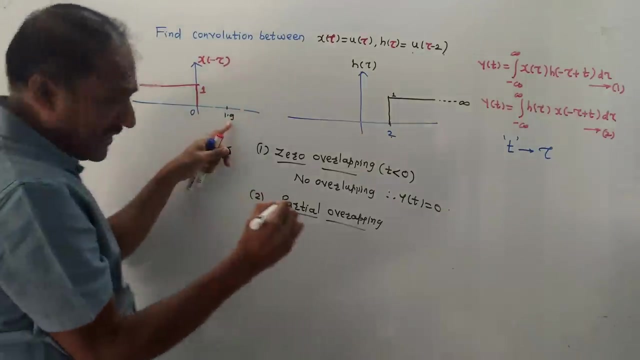 full overlapping condition. now i want partial overlapping. now this is a little different condition. partial overlapping, like i told you earlier, this diagram is shifting to right, but 1.9. if we shift till 1.9, then also there will be no overlapping minimum. we have to shift from 2. 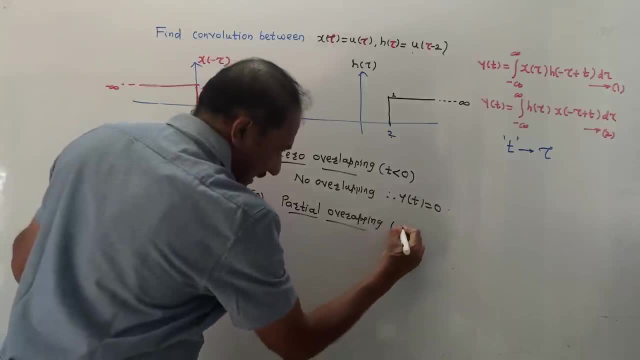 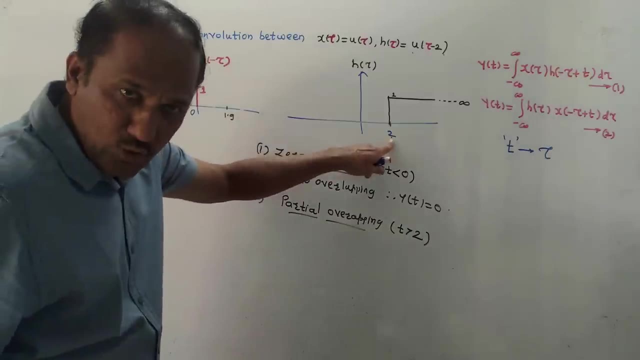 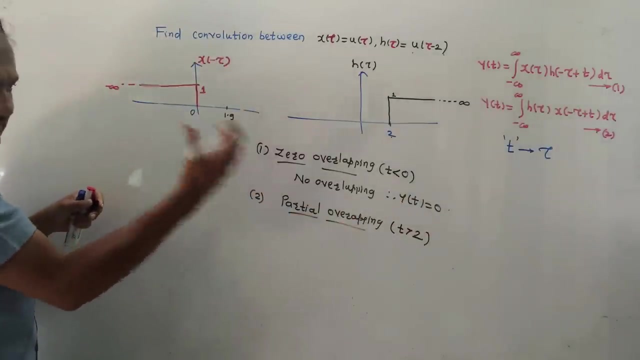 minimum we have to shift from 2. that's why in this condition bracket i will write t greater than 2. remember this: this diagram is starting from 2, so at least i have to shift till more than 2. then only there will be overlapping, otherwise there won't be any overlapping. 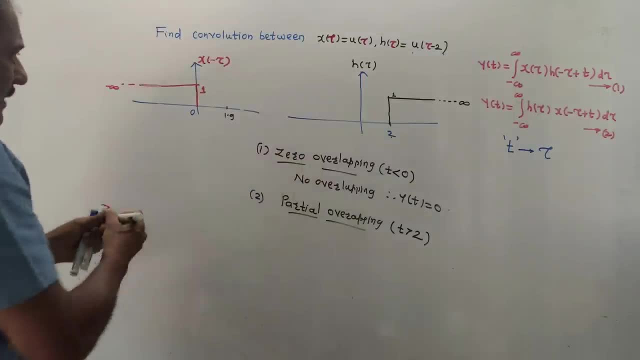 that's why i have written t greater than 2. i have to shift this diagram from more than 2. see now how to remember notations. this diagram is from minus infinity to 0. i have to shift this diagram from more than 2, from 3,4,5. 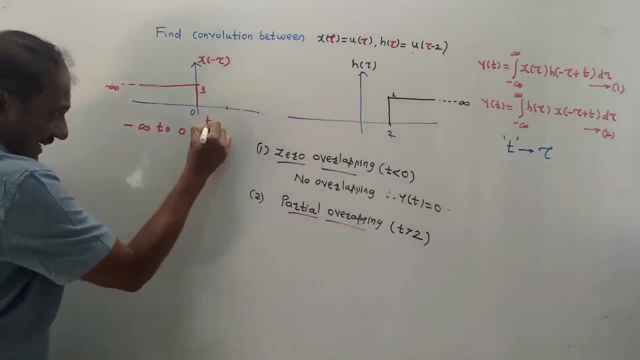 whatever, but think like this: shift from t amount and t is greater than 2 means how to write range. t is equal to 0. we have to add t in both. if we do minus infinity plus t, then minus infinity will be t. if we do 0 plus t, 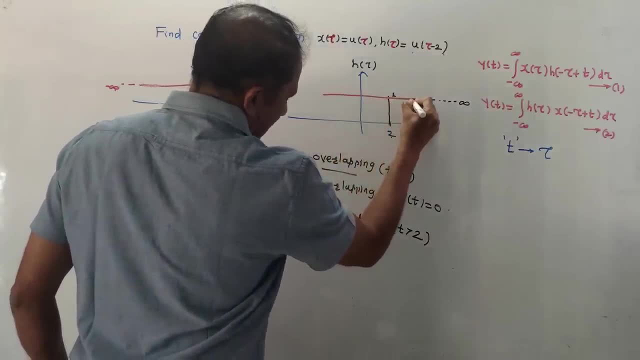 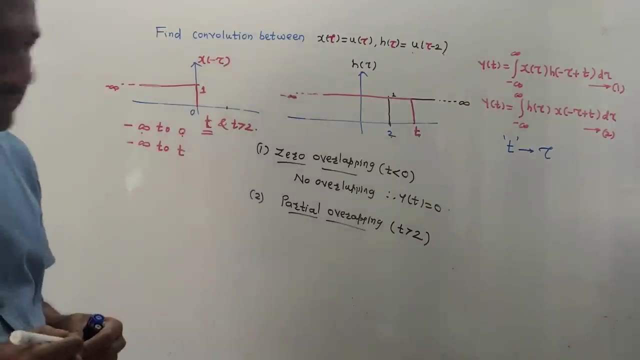 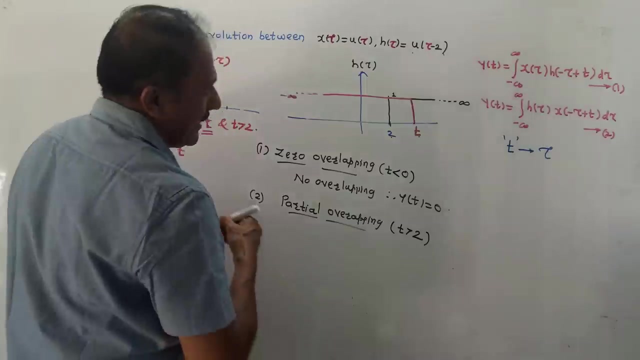 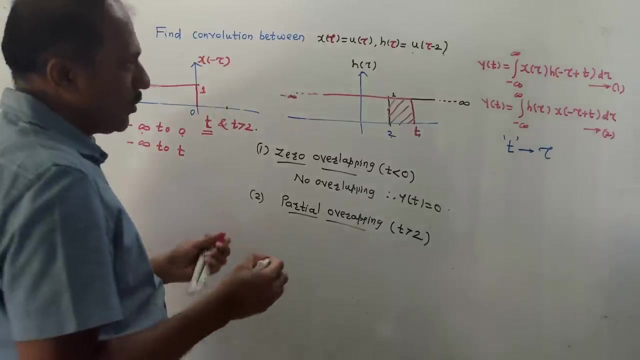 then t will come. this means while drawing new diagram. if we draw like this, it will come till t, where t is greater than 2, and this is from minus infinity, as we discussed last time. in this condition, so common portion is shading. this is known as overlapped portion. 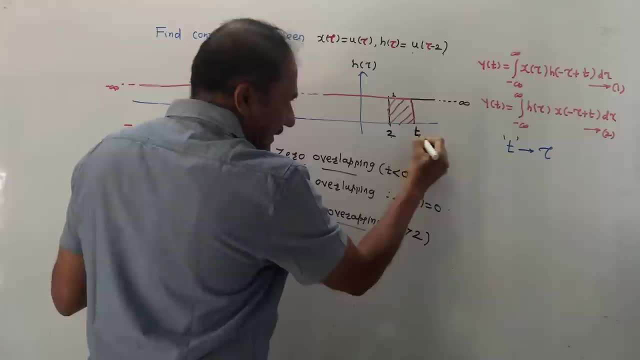 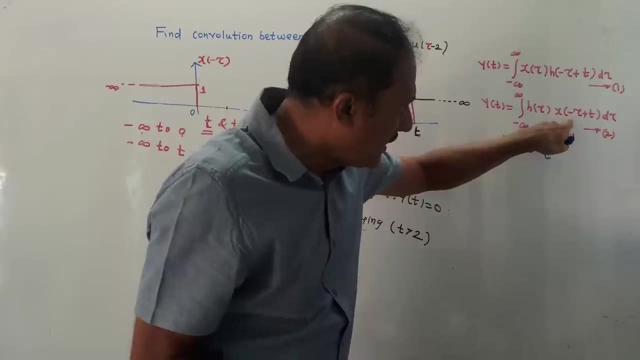 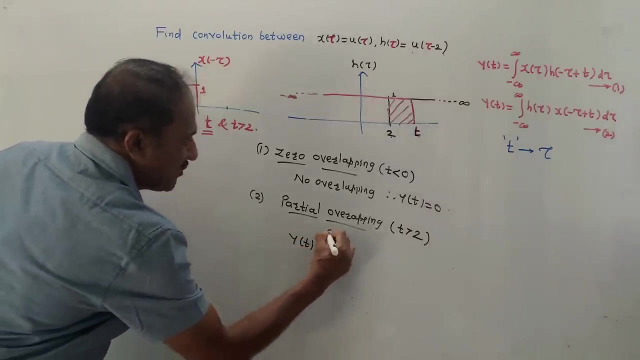 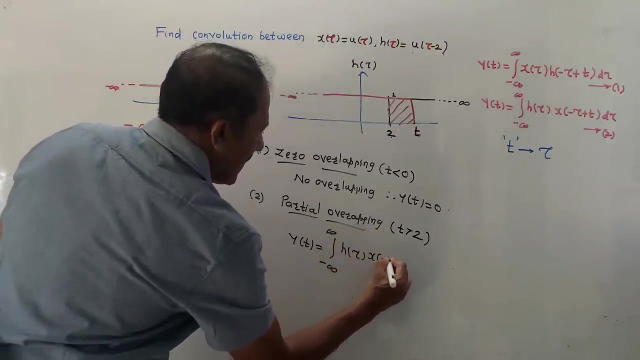 or overlapping. so from where to where is overlapping? from 2 to t. now we have folded x, so we have to use x, which is folded. let me write the formula. so it is: minus infinity to plus infinity, h of tau, h of tau x of minus tau, plus t. 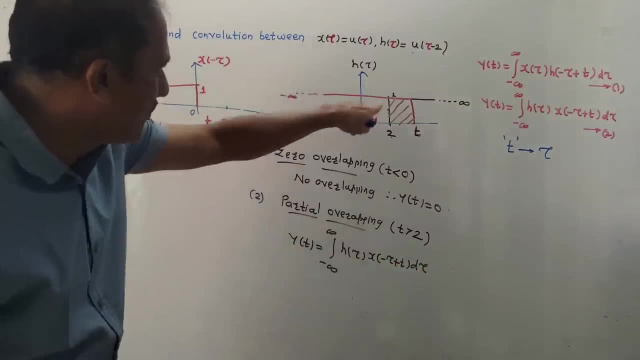 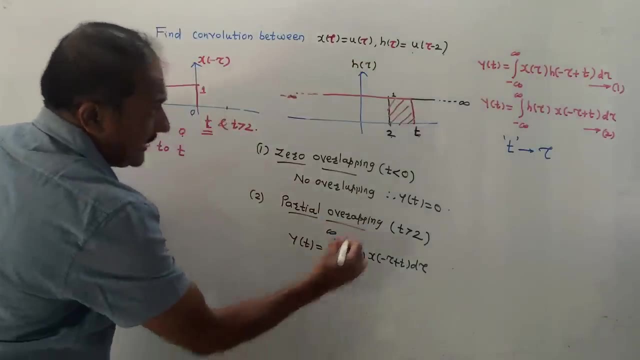 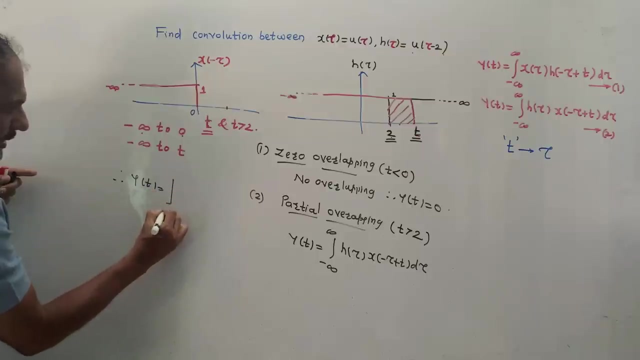 d tau. now we have to put values in this. h of tau means both are unit steps, so both values are 1. now how to change integration in this? from where to where is overlapping 2 to t? so i will write the new equation: y of t is equal to. 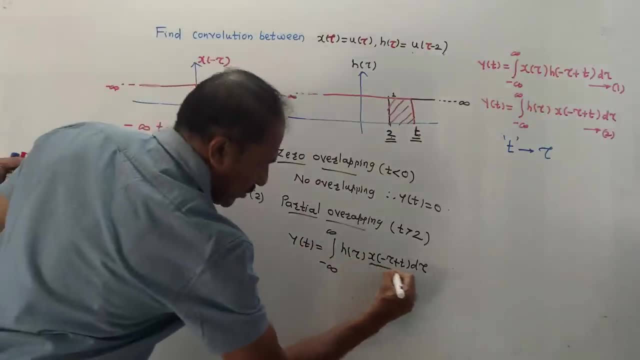 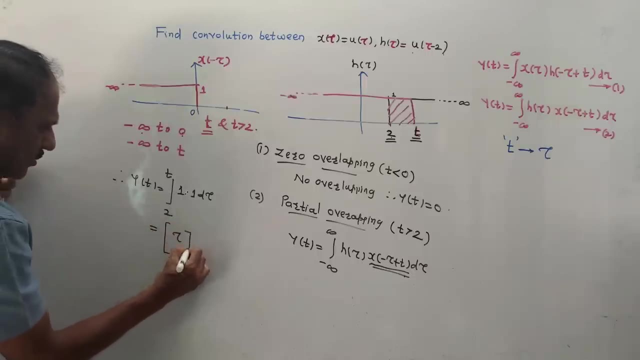 integration 2 to t. its value means amplitude, its 1 is second. this is also notation d tau. now this is simplest integration. integration of d tau is tau limits are 2 to t, put upper limit once, put lower limit once. so this is the final answer. 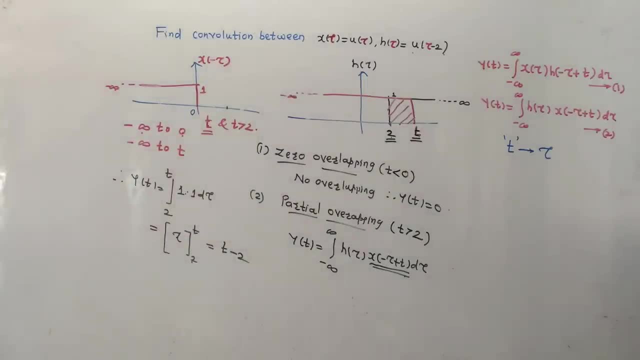 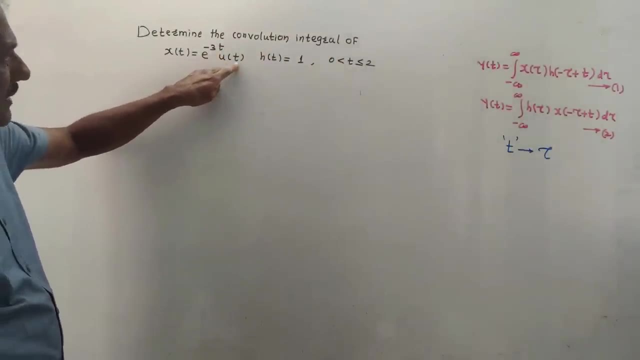 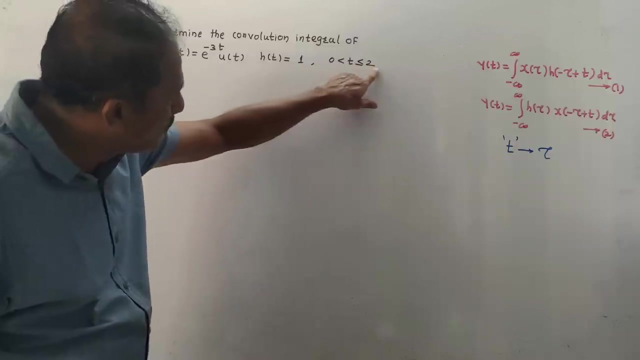 let us solve some different numerical next problem. determine the convolution integral of x of t. is e raise to minus 3t. u of t means this is exponential signal, like the numerical number. 1 is between 0 to 2, because 0 is less than t. 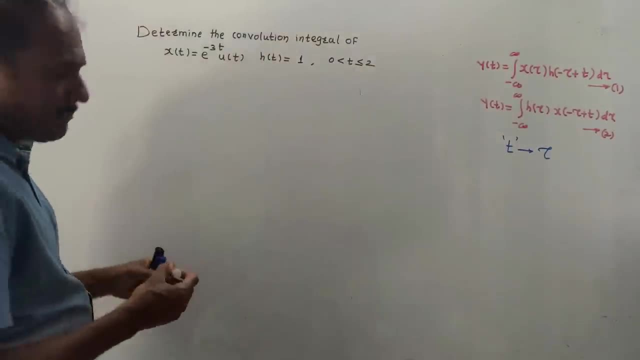 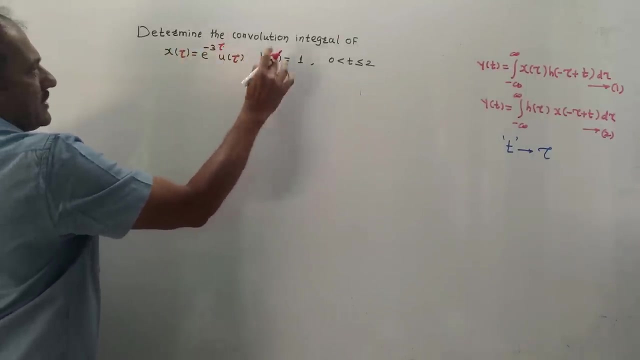 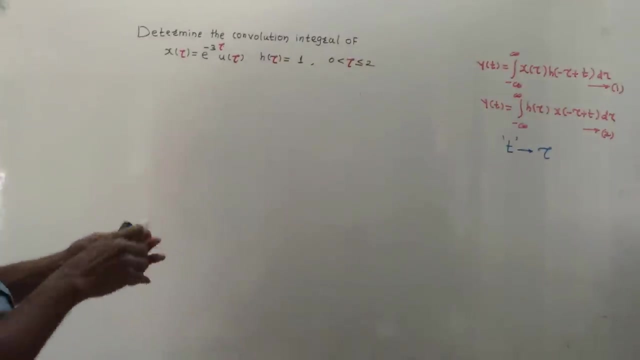 is less than equals to 2, as usual in every sum. first step is to replace variable t by tau. write the new equation. so i am just replacing the variable. replace t by tau, simple. now let us draw both diagram. first signal is x of tau, which is e raise to minus. 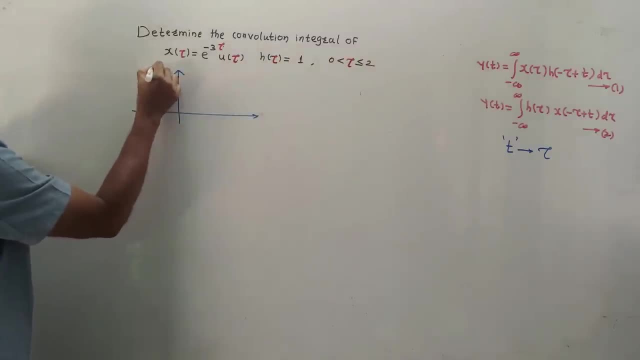 3 tau. u of tau in the first numerical we have drawn. it is exponential signal, i have already explained, and u of t is multiplied. so this whole signal will come in positive side. so diagram of signal is like this: this is still infinity. its value is e raise to minus 3 tau. 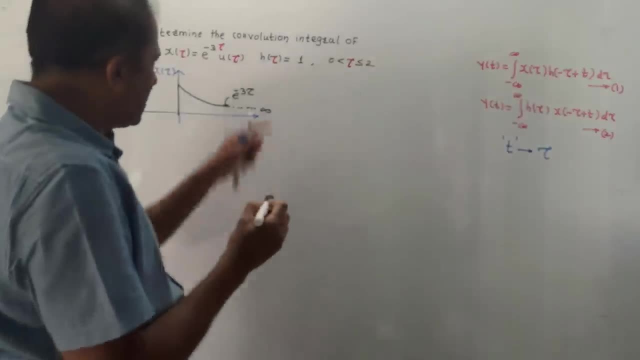 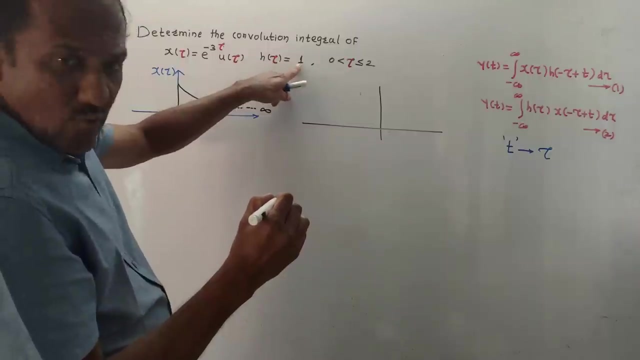 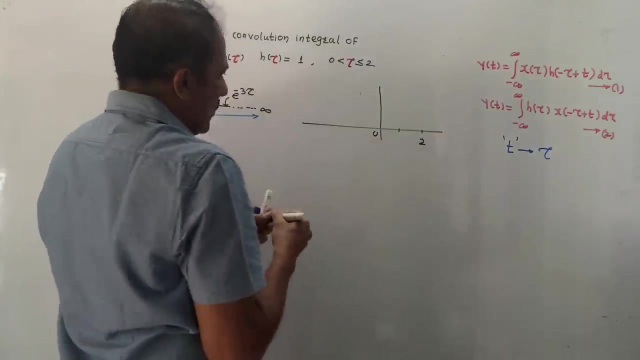 now second signal. i have to draw h diagram. see h diagram. this is 1. from where to where? from 0 to 2, i mark scale. this is 0, this is 1, this is 2. 0 to 2 is its amplitude 1. 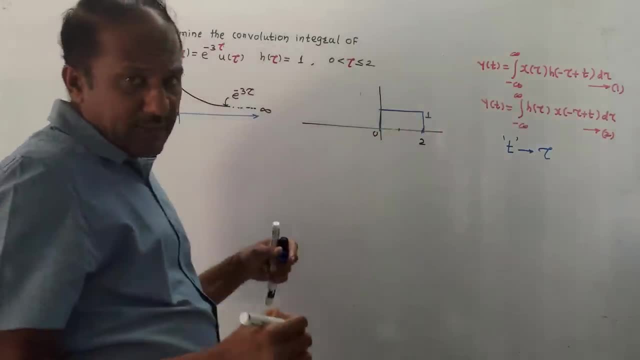 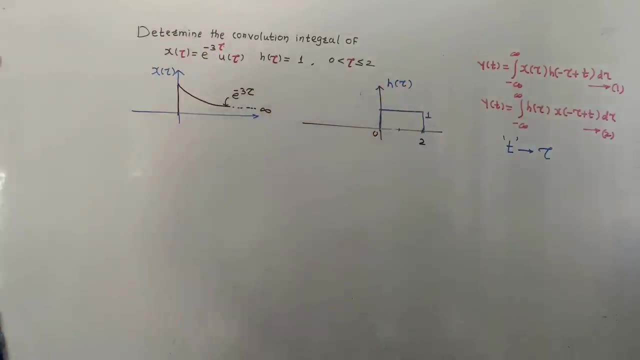 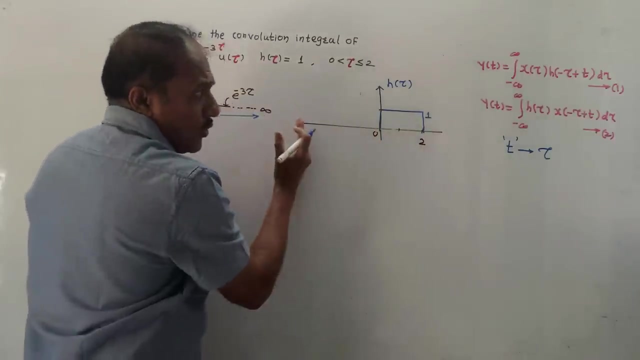 so diagram will be like this. as i told you, diagram will not be given in the question. you have to make diagram. this is signal of h of tau. now we have to think which fold will be simple. we will fold that. naturally this looks more simple. its fold means in mirror image. 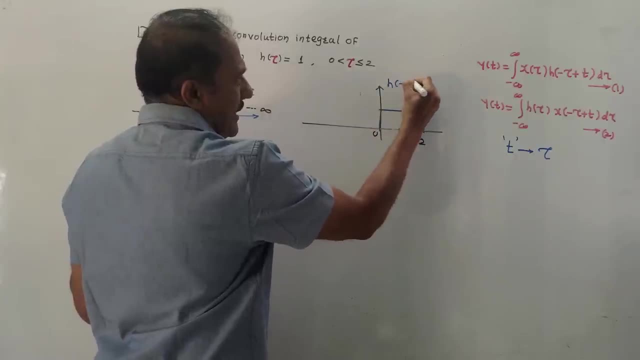 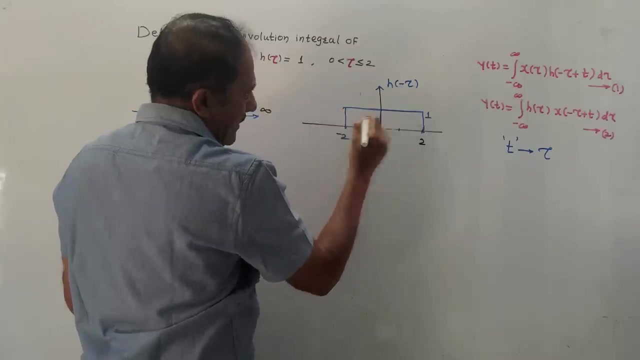 this will be in positive side and this will be in negative side. so i will do h of minus tau. and in negative side means it will come till minus 2. this amplitude will be as it is and i will rub out this. this is the diagram of h of minus tau. 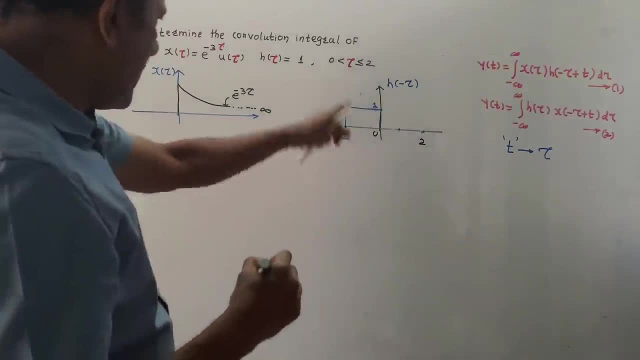 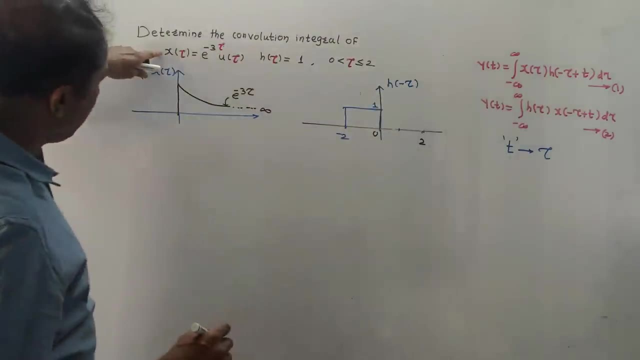 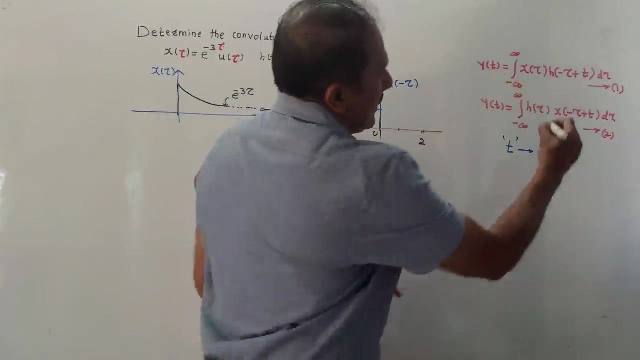 whose amplitude is given in 1 question. so i have drawn both the diagrams. one is signal as it is, second one is folded. now we have to think this: we have folded h, so i will be using equation 1, in which we have h of minus tau. 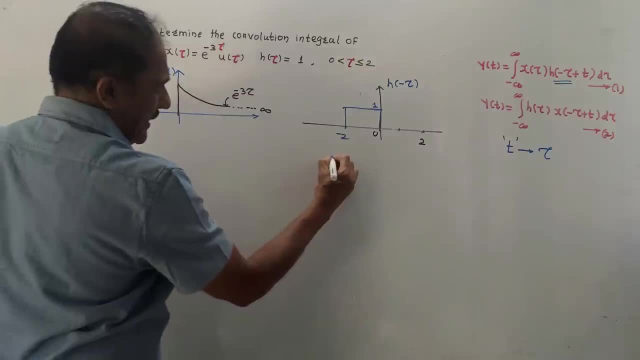 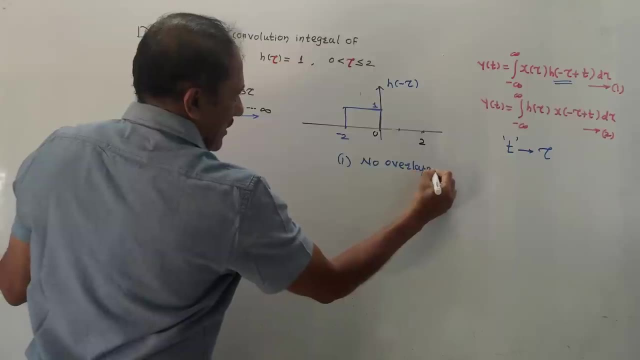 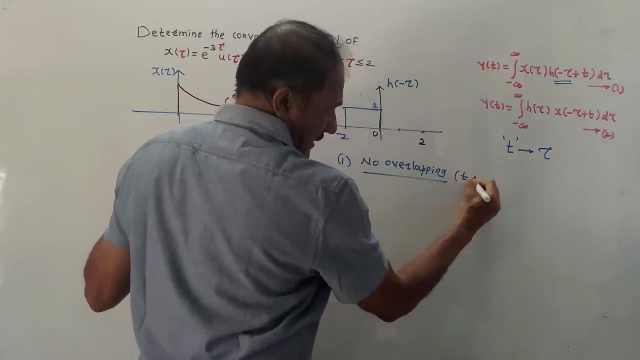 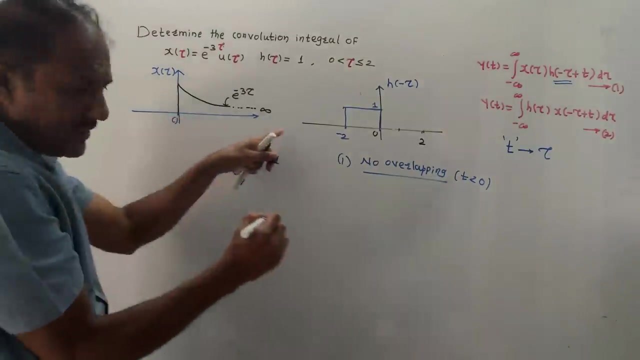 now, like the previous case. first condition: no overlapping or 0 overlapping. think like this: like every numerical, see how fixed it is, how simple it is. t less than 0 means if you shift left, then only it will not be overlapping, because this whole diagram is from 0 to infinity. 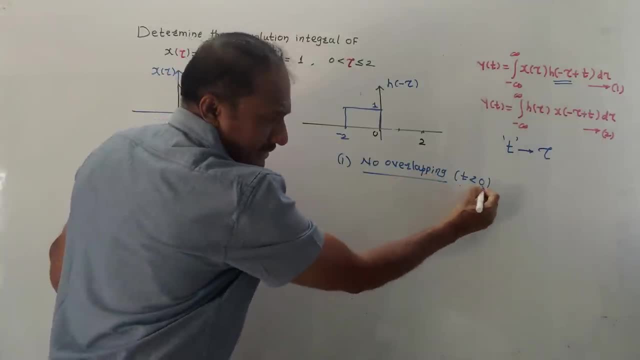 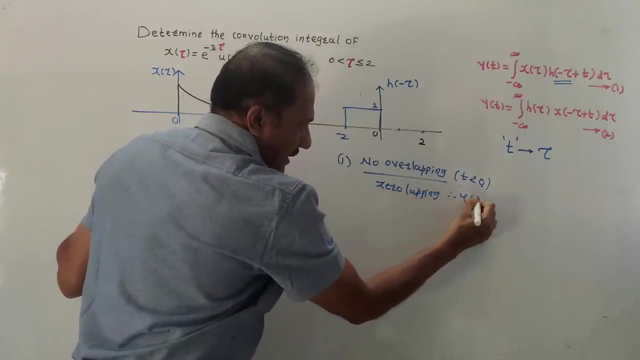 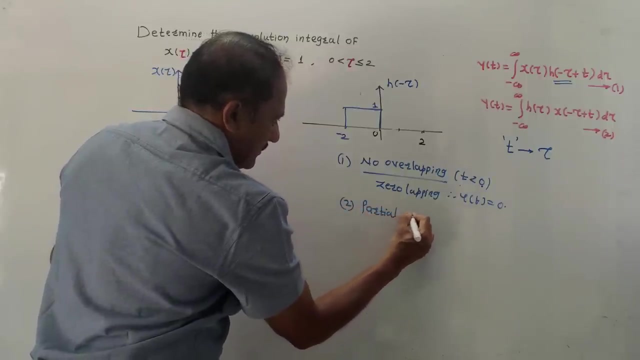 so i will have to shift it towards left. that is why i wrote t less than 0. here i have to write 0 overlapping, like all sums, and y of t is equal to 0. second condition: partial overlapping now see. partial overlapping means we do not have to overlap. 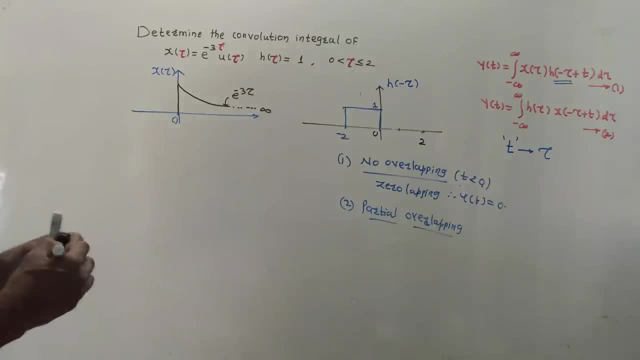 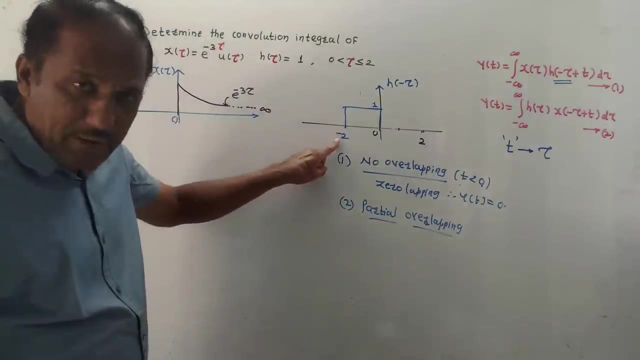 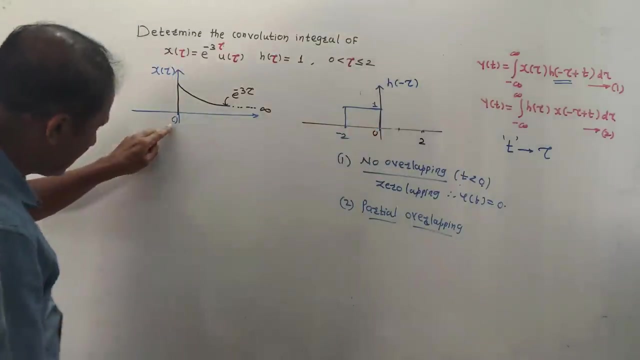 the whole signal. we have to overlap a part of it. now, how to think about this? think like this: this signal is minus 2 to 0. think like this: we have to discuss partial overlapping. when can we get full overlapping? one signal is from 0 to infinity. 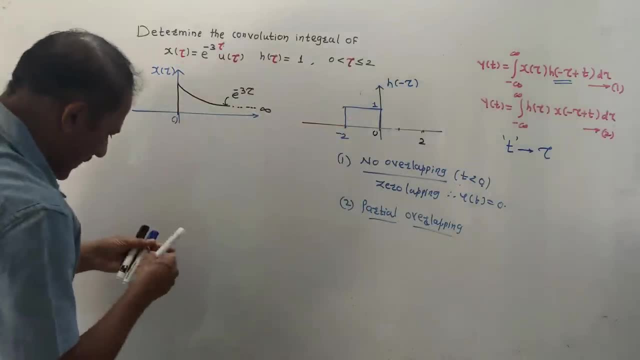 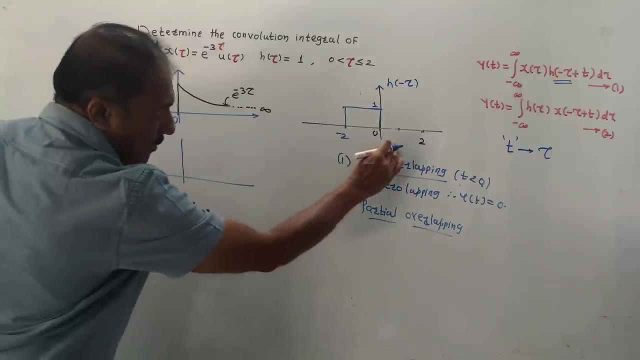 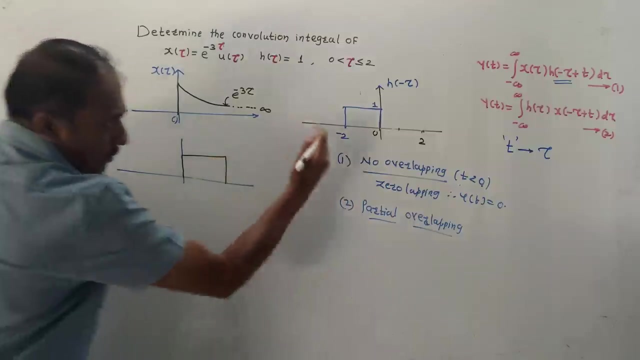 if i complete this, suppose i will draw one diagram for explanation purpose. this diagram: if i shift right with 2 amounts, if i shift right with 2 amounts, then signal will be from 0 to 2. like this: i am shifting right with 2 positions. 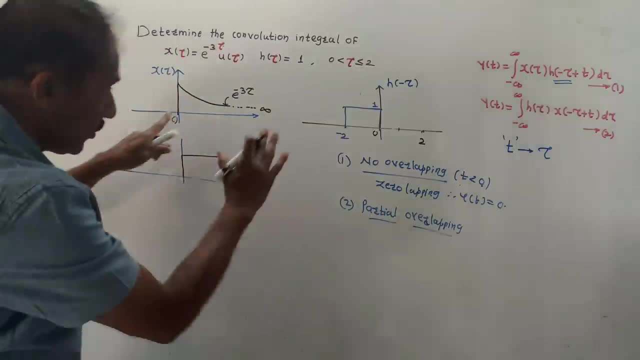 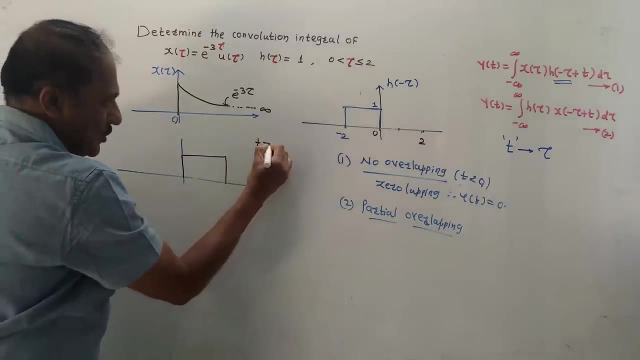 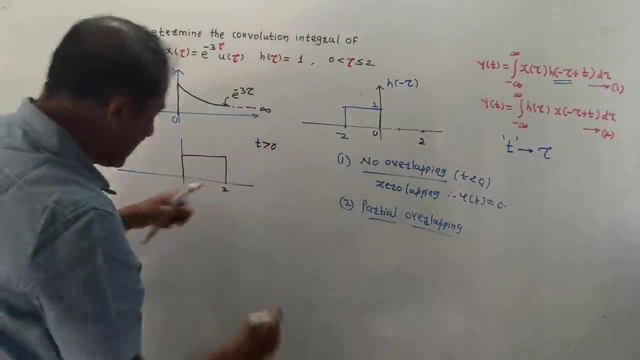 this is full overlapping. i want partial overlapping. what does this mean? one thing is clear: we have to shift right because this whole diagram. we have to shift right means t greater than 0, right means t greater than 0. for example, if i shift right with 1 position. 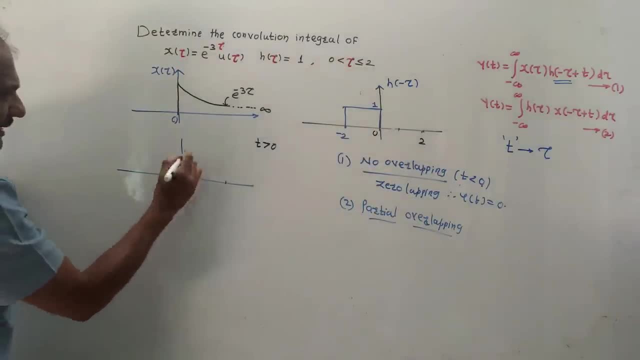 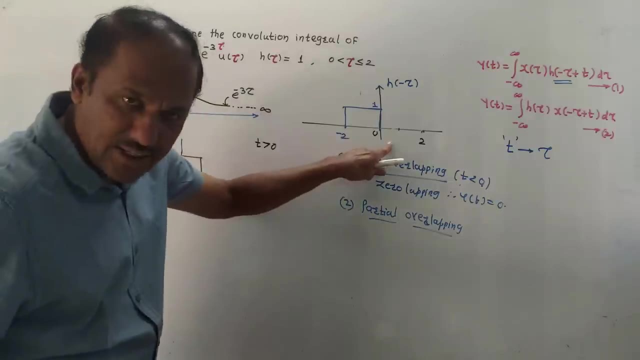 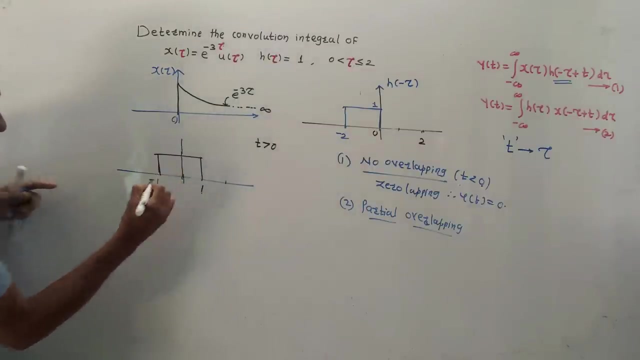 then from where will the diagram come? if i shift right with 1 position, then the diagram will come from minus 1 to plus 1. if i shift right with 1 position, then from minus 2 it will come from minus 1, from 0 it will come from 1. 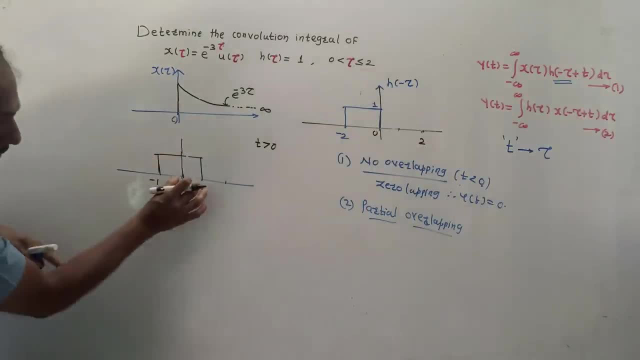 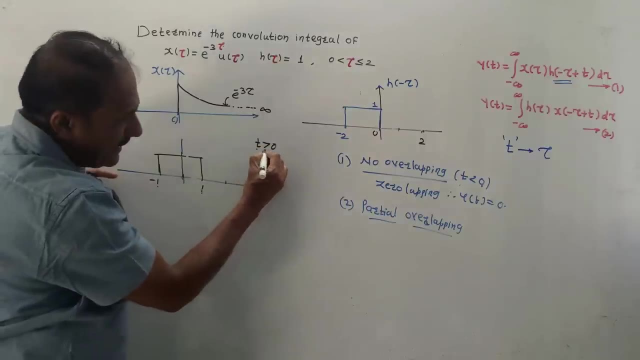 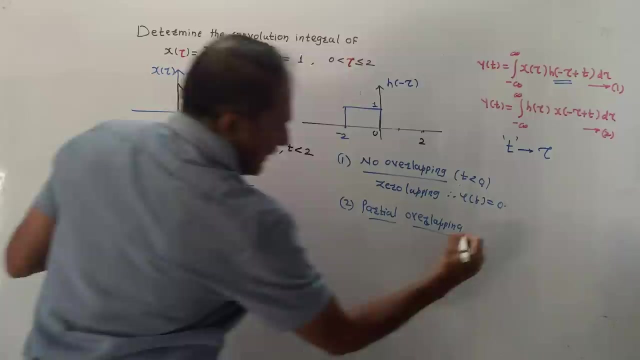 so here it is minus 1 to plus 1. this is partial overlapping. so while writing condition how to write one is to shift right. so t greater than 0. second t should be less than 2 means how to write combined condition 0 less than t. 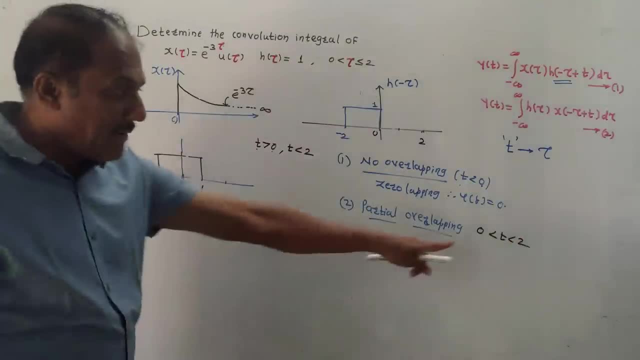 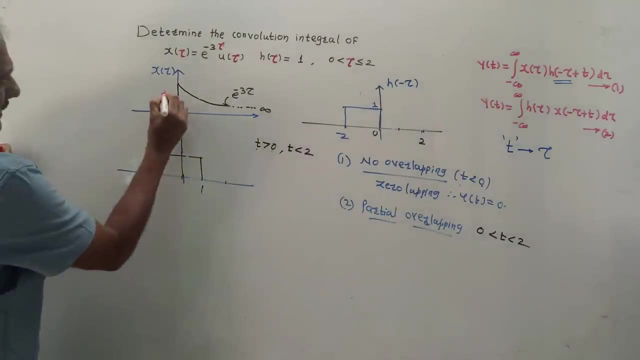 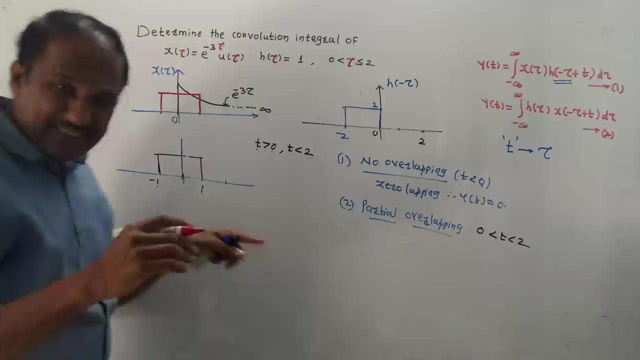 because t greater than 0 is 0 less than t and t less than 2. this is combined condition for partial overlapping. now in one diagram it is like this: now most important part: this is minus 1 and plus 1 means. i have used this to understand. 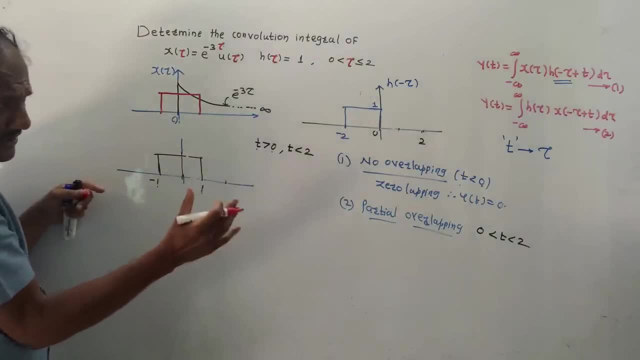 always remember this notation is required in tk terms and range. we have already written: t is between 0 to 2, that is, 0 less than t less than 2. so minus 1 and plus 1 should not come like this very simple technique i say. 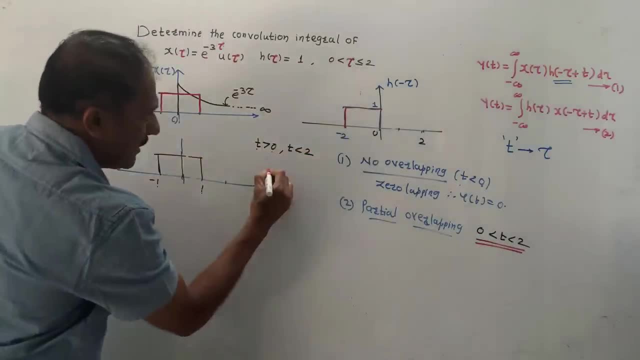 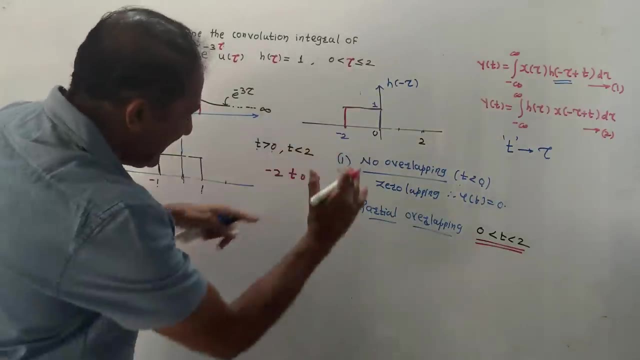 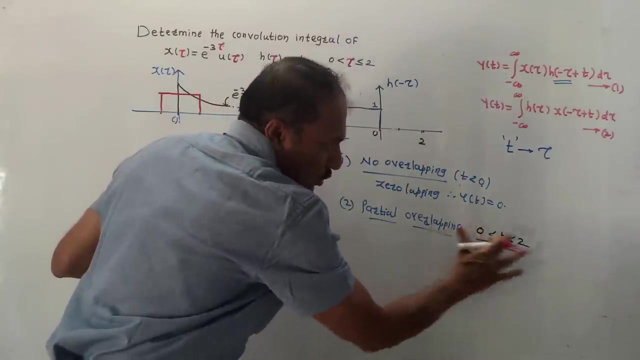 this original diagram means the diagram we have to fold from where to where. ok, now to write in notation terms. make it more simple. i have to shift right by amount t and t will be 0 to 2 once you have written range. after that it is not thinking about 0 to 2. 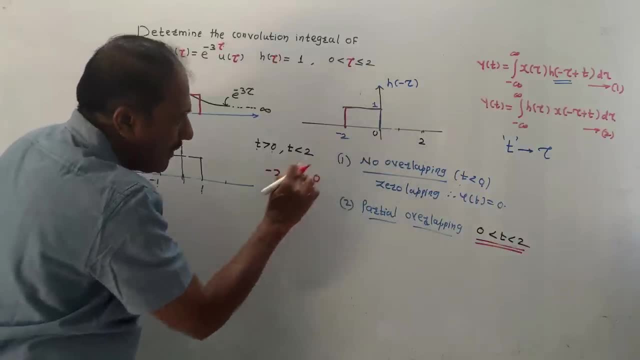 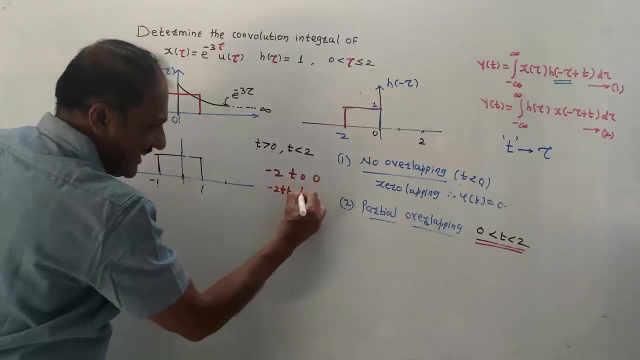 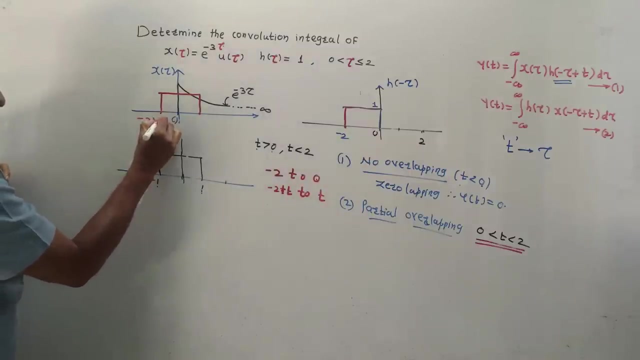 so what to do? this is minus 2 to 0. this is original signal which is folded. we have to shift from t, so i will write new limit: minus 2 plus t and this will come to t. now from where to where overlapping comes? overlapping means common portion. 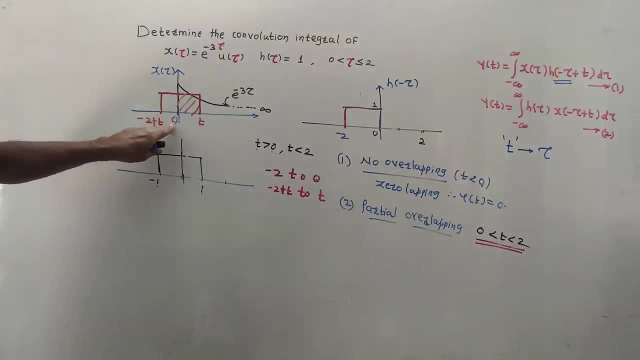 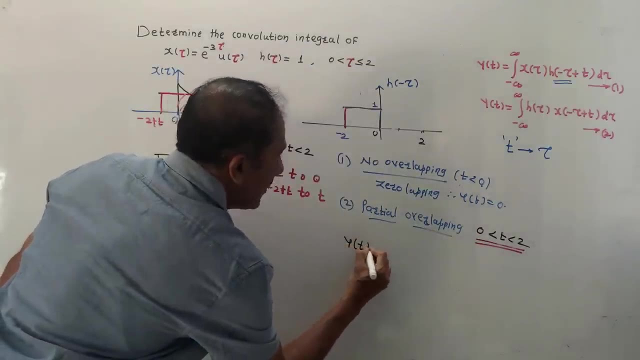 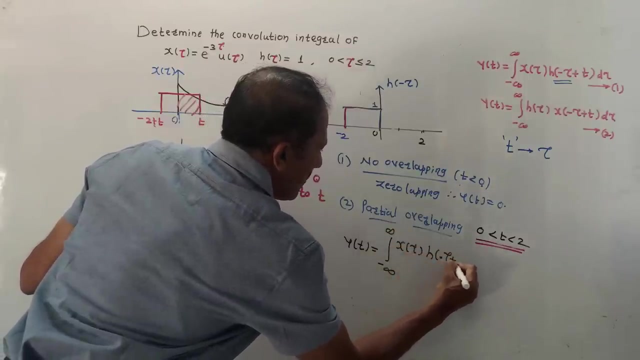 overlapping comes from 0 to t, from 0 to t. now first i will write the formula of integration y of t is integration minus infinity to plus infinity, x of tau, h of minus tau plus t d tau. now think like this: from where to where overlapping comes? 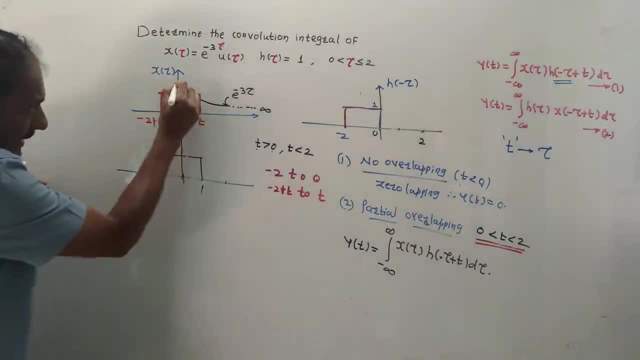 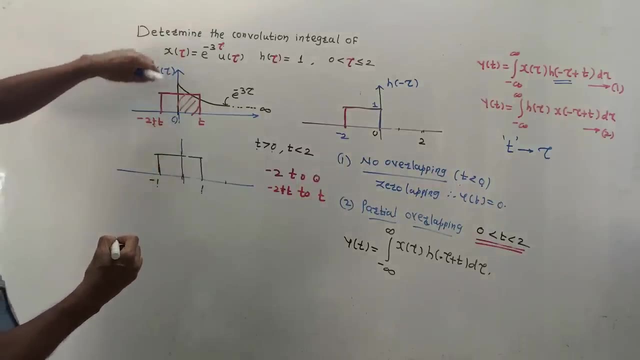 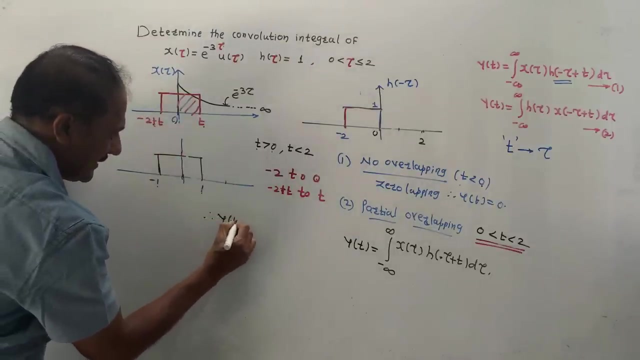 from 0 to t. overlapping means common portion. this first signal of x is in right hand side, second is in left, but this left one is of second signal. there is no part of first signal. overlapping is common portion. so range will be 0 to t. so in this case i will get it like this: 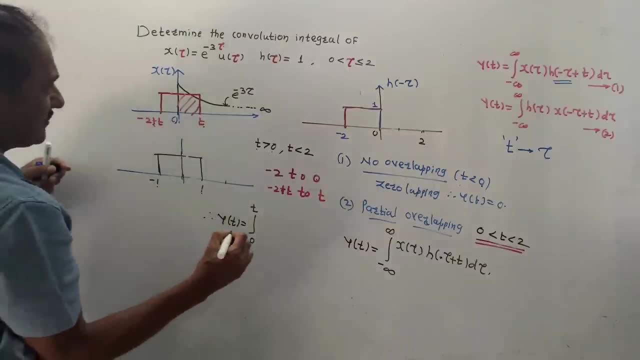 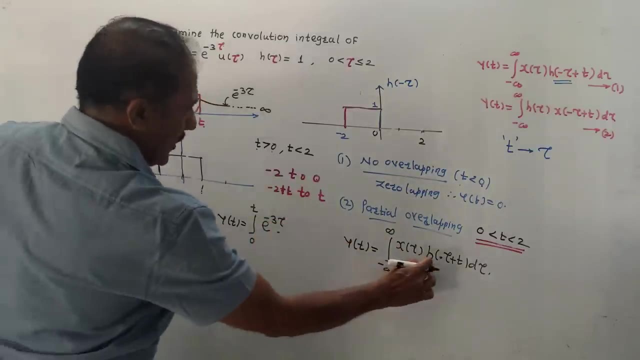 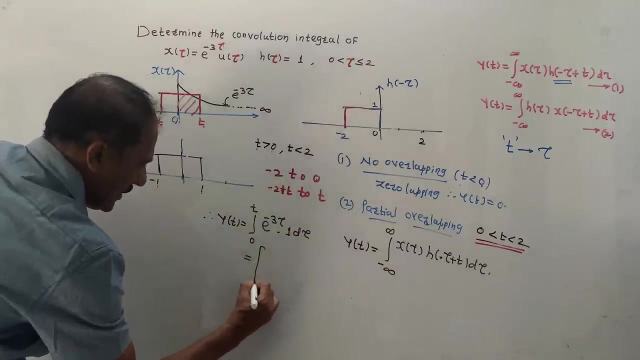 integration 0 to t. now value of x. x means this signal, e raise to minus 3 tau into h value. value means amplitude. amplitude of this is 1. is t tau. very simple. now only integration has to be solved. so it is e raise to minus 3 tau. 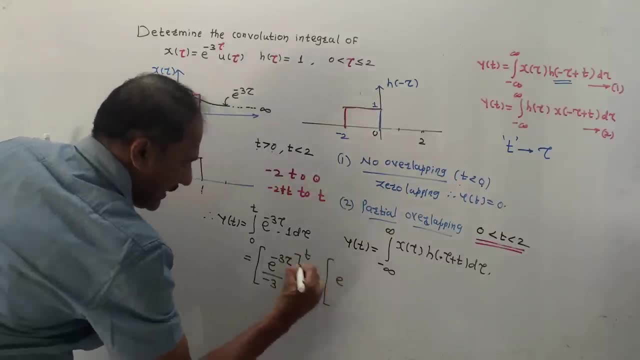 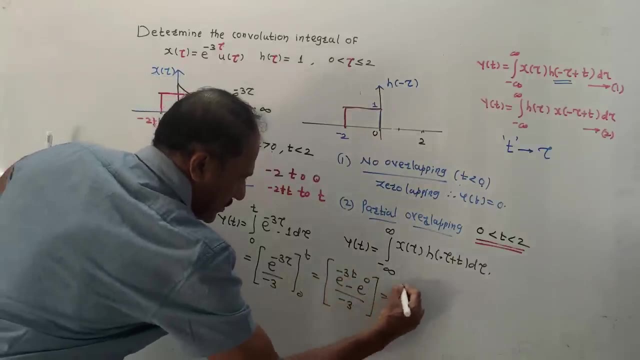 upon minus 3. limits 0 to t. simplify it: first put the limit on you e raise to minus 3. t minus e raise to 0 upon minus 3. e raise to 0 means 1, so it is e raise to minus 3 t. 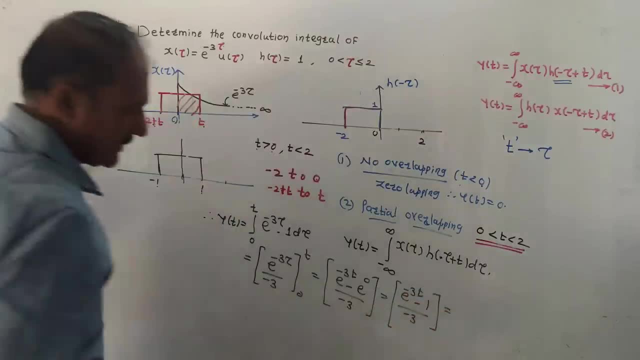 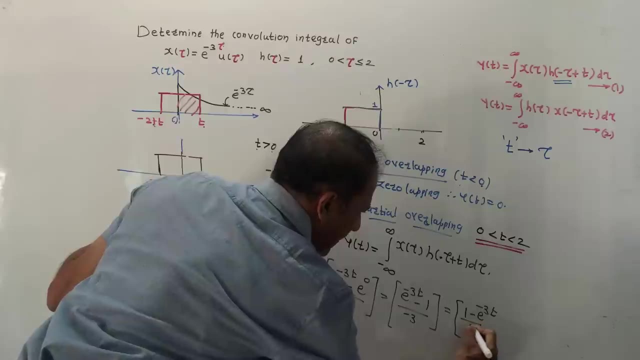 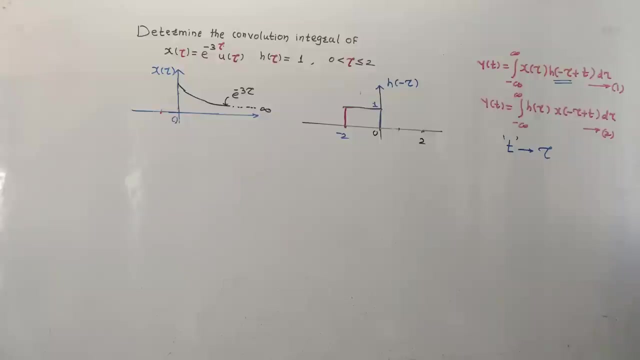 minus 1 upon minus 3. and next step: you can do, you can solve this minus sign. so it is 1 minus e. raise to minus 3: t upon 3. this is the condition of partial overlapping and one more condition is left, that is full overlapping. 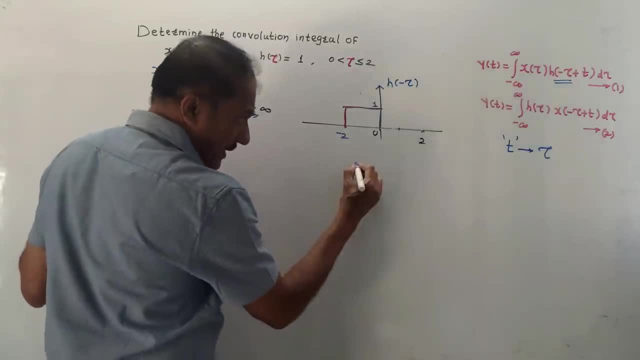 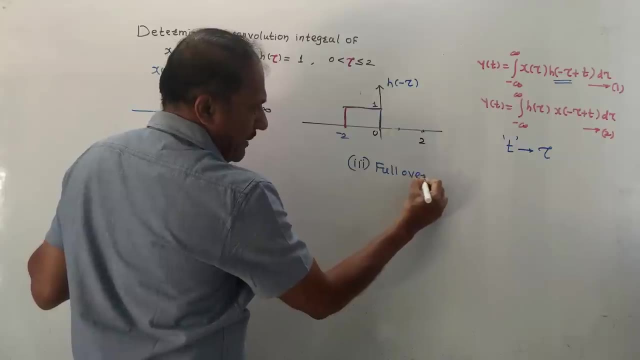 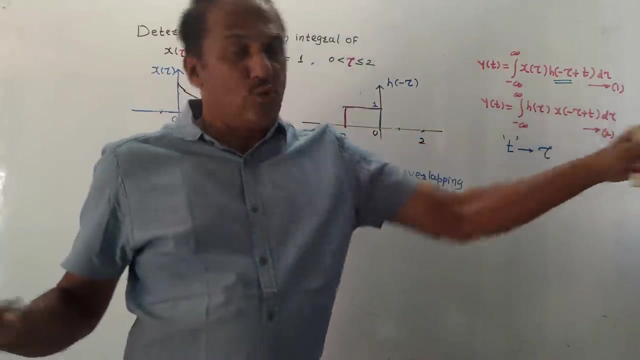 now third condition. first in two numerical. there is no condition. in this numerical there is condition. so third condition is full overlapping. full overlapping means I have discussed in two numerical: if two signals are overlapping till infinity, then we have to consider. but if one signal is finite, then full overlapping means. 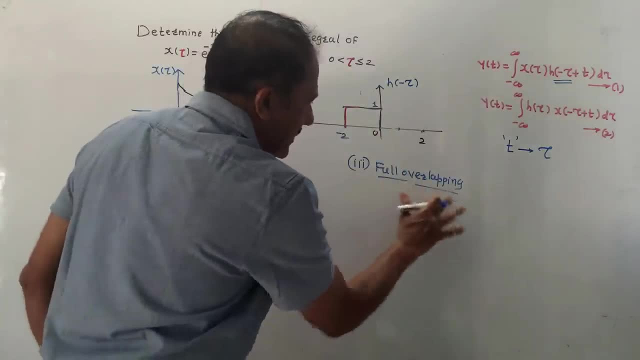 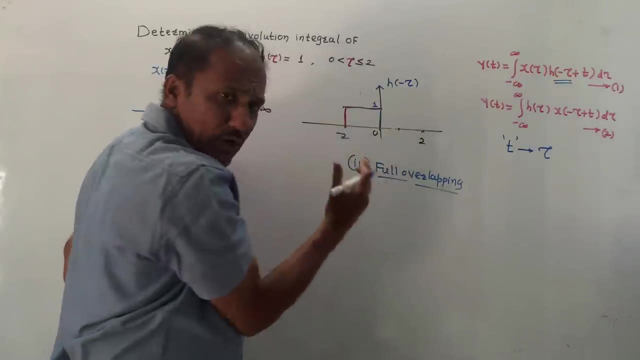 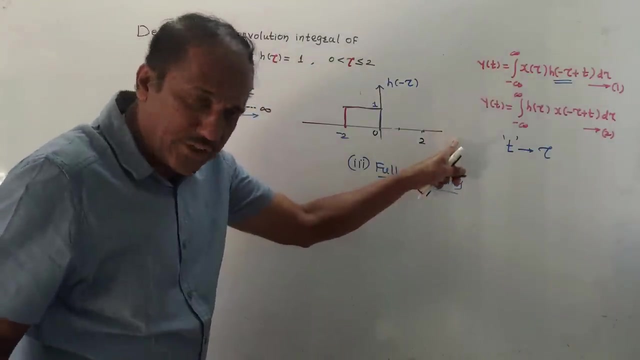 only finite portion will be overlapped. so we have to consider this condition now how to think? I have just explained the concept. if we shift from 2, then it will be full overlapping more than 2, no matter how much we shift. for example, I shift from 3 to right. 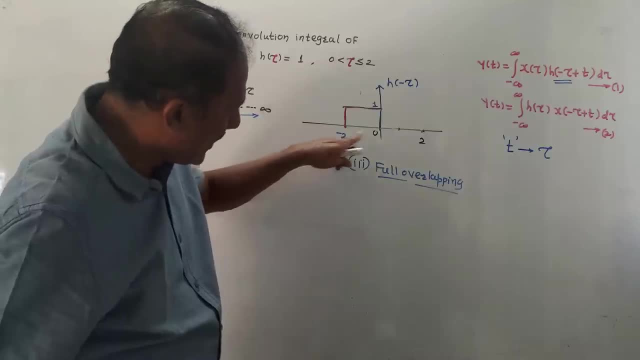 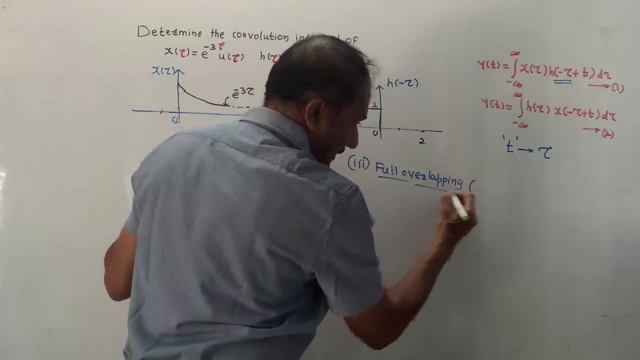 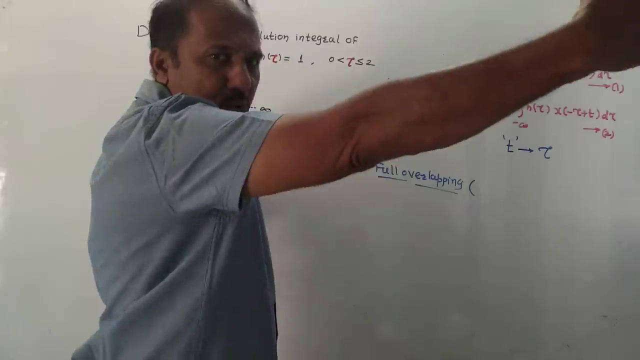 so if we shift from 3, then it will be minus 2 upon 1 and 0 upon 3, so it will be full overlapping like this. now how to write the condition mathematically? how do I know? if we shift from 2 then it will be full overlapping. 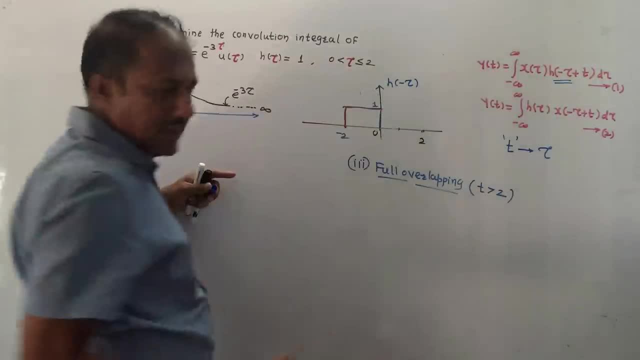 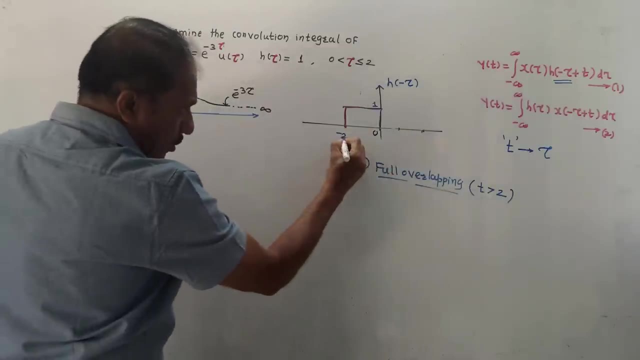 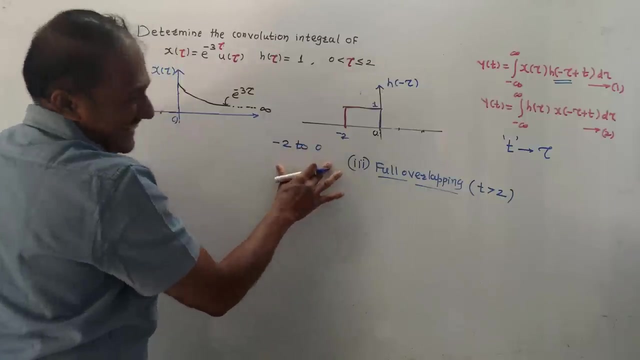 no matter how much we shift, then it will be full overlapping. so in condition bracket we have to write t greater than 2. this original signal from where to where is from minus 2 to 0. in this we have to add t because we are not shifting. 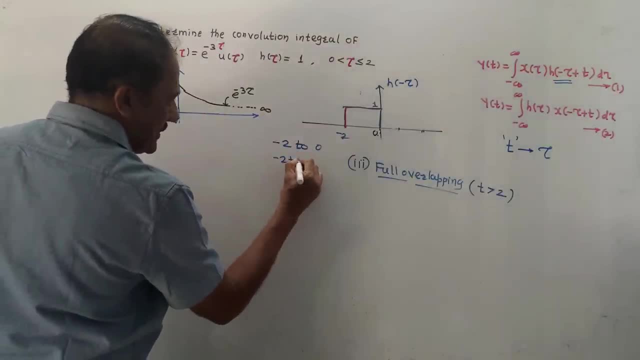 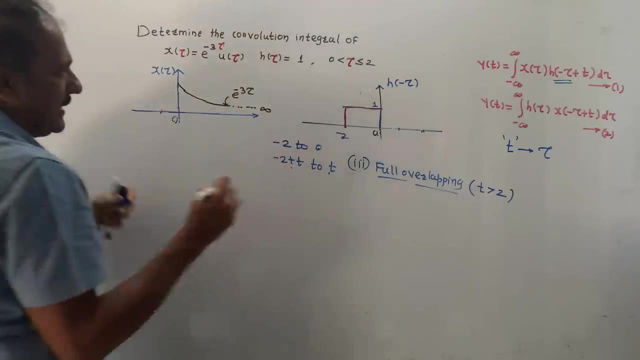 from fixed amount. we have to shift from t only, so it will be minus 2 plus t and from here it will be 0 plus t. we have to add t in this. now, in the same diagram, we have to draw two signals, but this is 1 and this is 2. 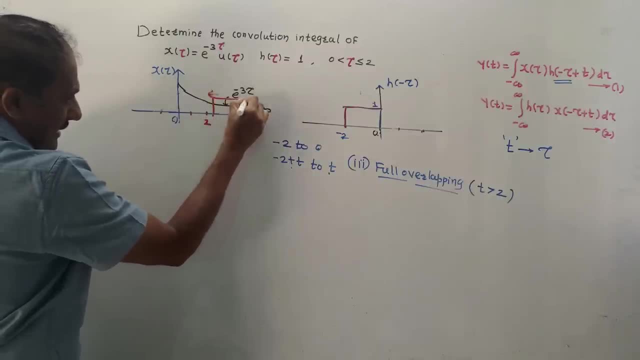 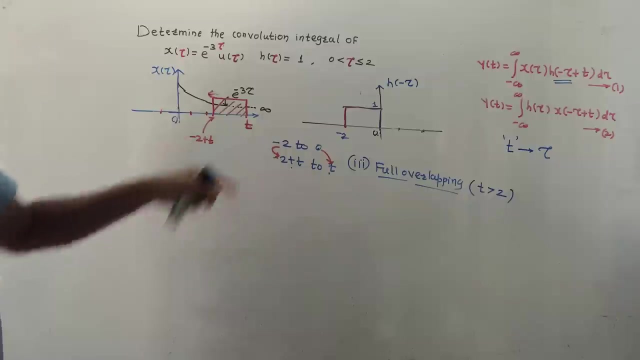 so I draw two signals like this, like this: this is full overlapping. here I have marked after 2. here I have to write minus 2 plus t. I have explained: here I have to write t. so overlapping means common portion will be from minus 2 plus t to t.